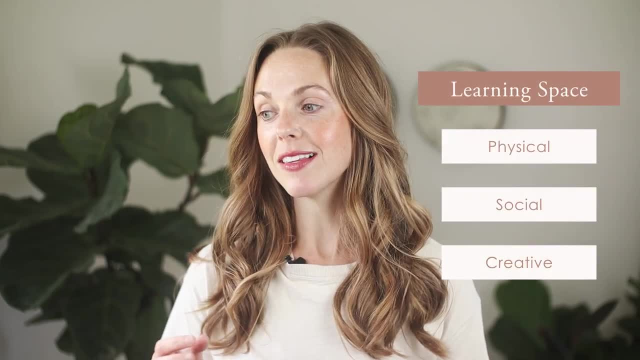 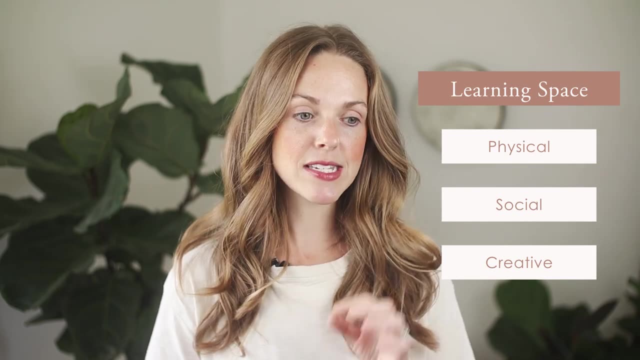 learning space as a whole, And that's going to include things like the physical space, right? So how do I move my body and how do I move my body around the room? We're also going to want to set some expectations for the social space, because all of our learning experiences are 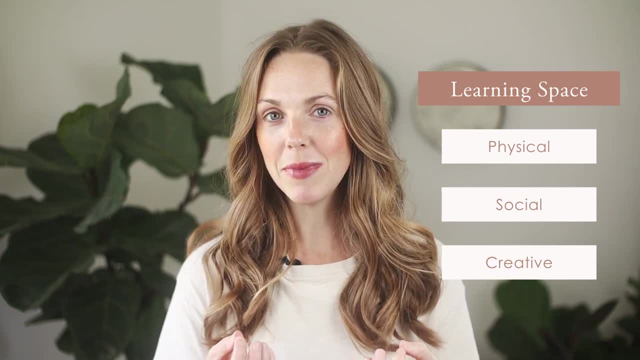 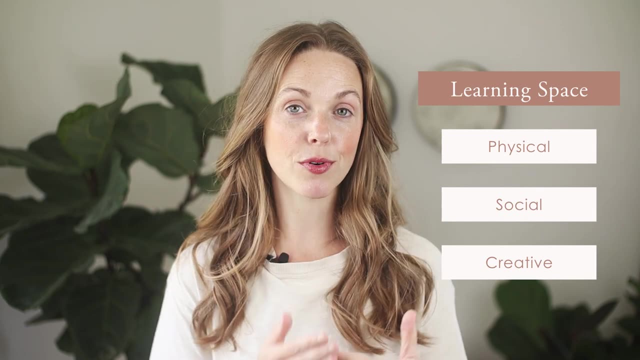 going to happen in an interdependent ensemble. So what does it mean to be an active member of that musical community, of that musical ensemble? We also want to start thinking about the creative process in learning. So how can we invite some creative thinking on the very first day? 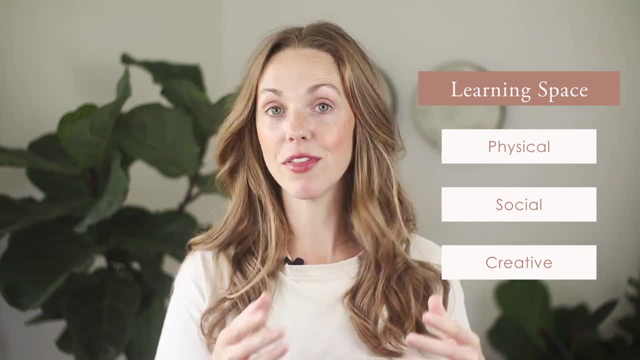 but still in a safe way. So, to that end, let's look at a couple of things. Let's look at a warmup routine, Let's look at a welcome song, Let's look at a getting to know you activity and a name. 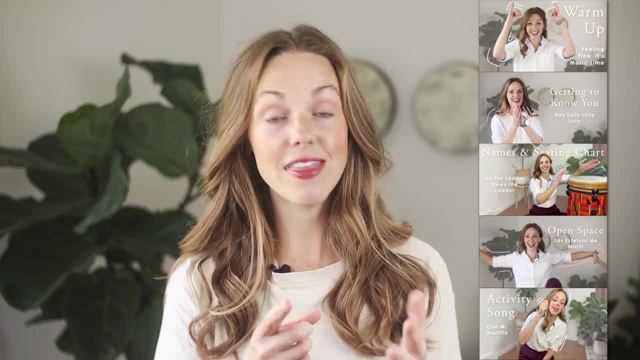 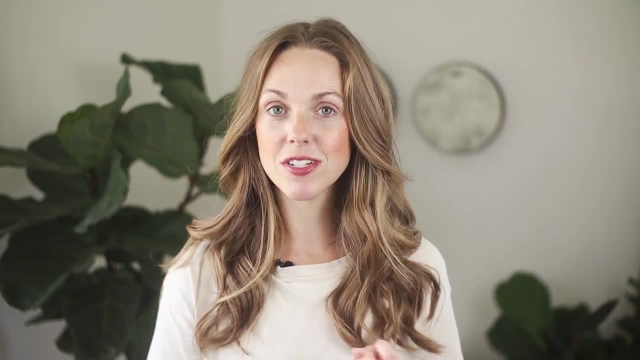 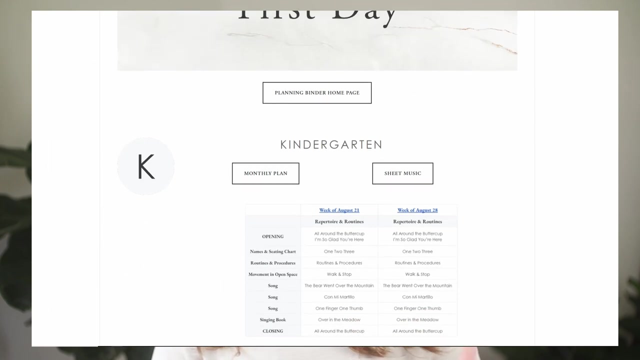 And then let's look at an activity for open space and then an action song. So a lot that we're talking about here. All of the videos that we are using today are from the first day resources and the 2023, 2024 planning binder subscription. These are long range plans, like a scope and 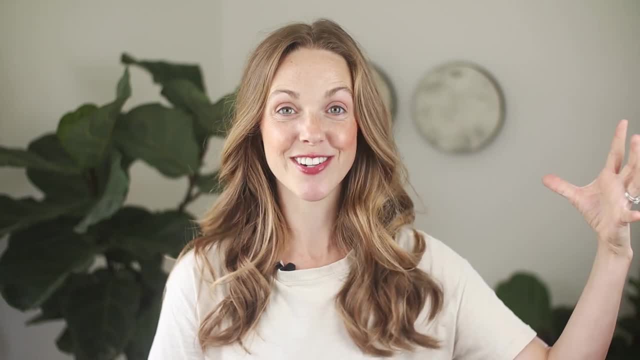 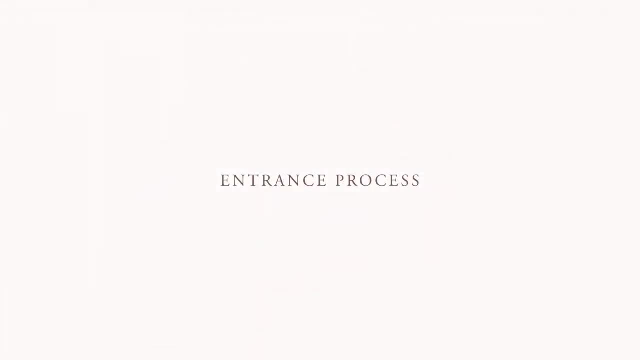 sequence, like song lists, things like that, The very big picture of the year as well as first day activities for kindergarten through upper elementary, including older beginners. Let's start with the class entrance, the warmup routine and the welcome song. These are two. 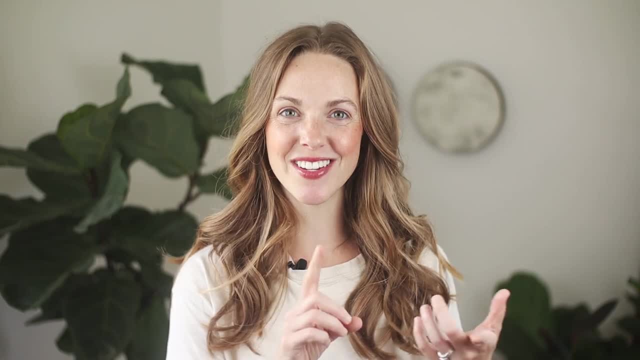 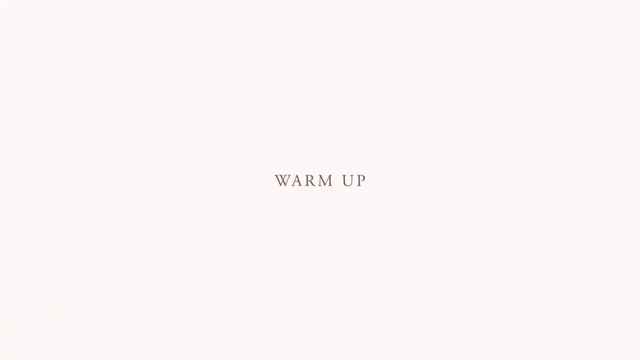 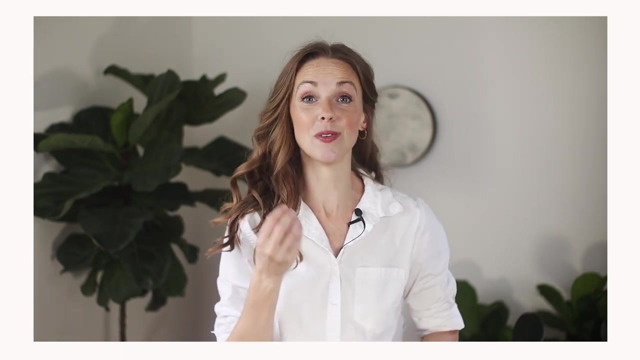 composed songs They happen to be. the first one is in Dorian, The next one is in Mixolydian. So kind of a fun way to start the first experiences in elementary general music In our first moments of class. in the beginning of the year and beyond we have a couple of goals. 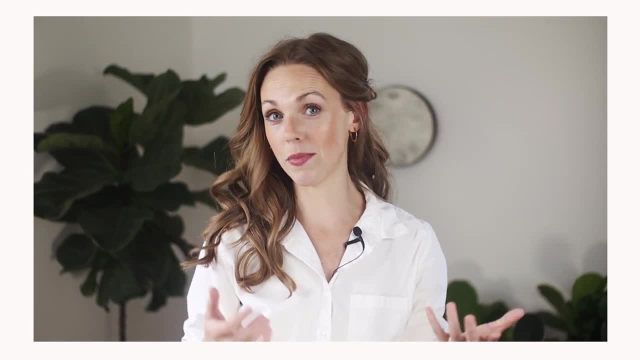 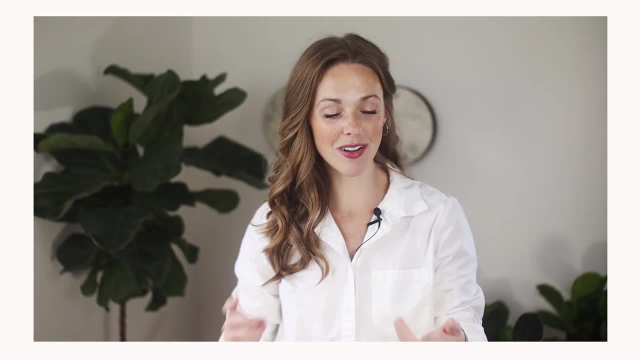 that we want to start working through for our warmup routine. One of them is just simply getting students from the beginning of the year to the beginning of the year. So we want to start working from the hallway and into the music class in some sort of a safe and orderly and musical way. 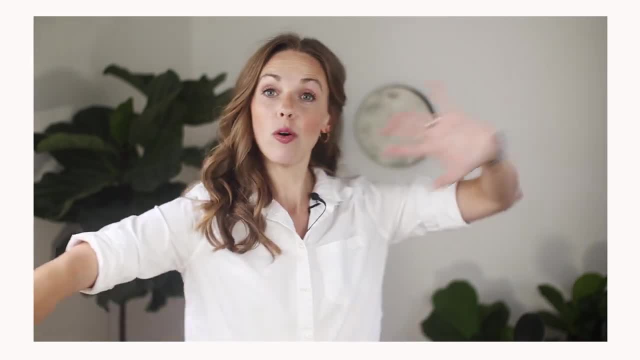 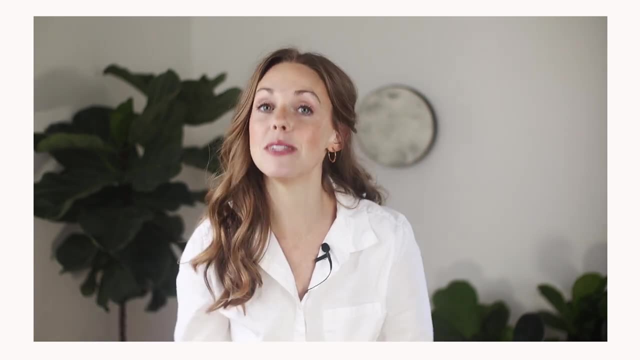 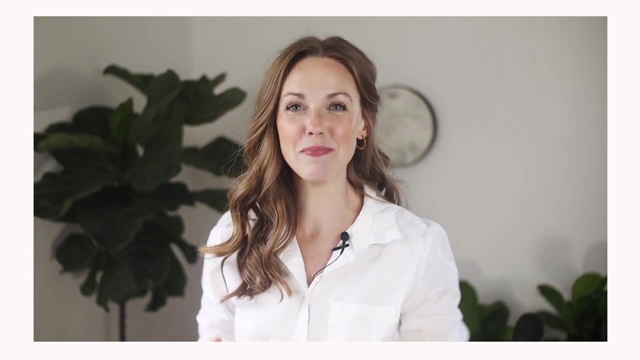 Once we're there, we're going to go through some body awareness type activities where we get to do some stretching, some mirroring. We can transition that from some steady beat motions, depending on where students are in their kind of physical development of the beat. That will be really. 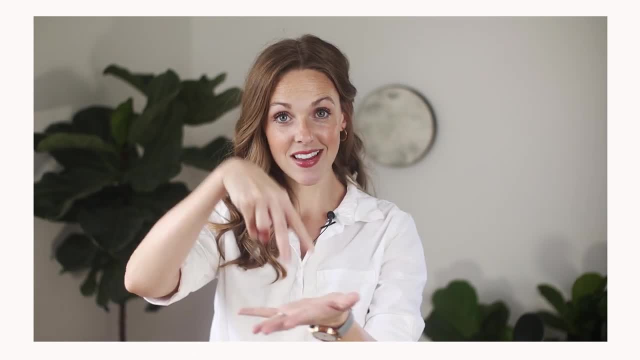 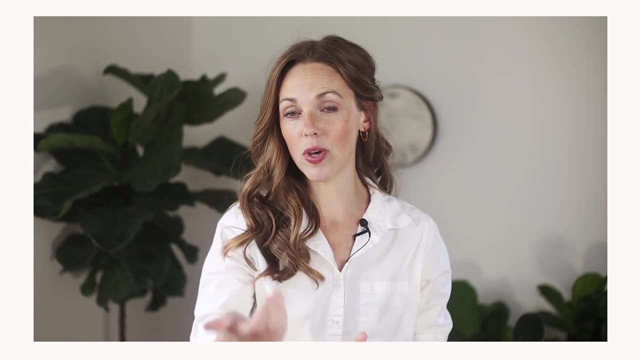 good for us to see. We also want to do some signs for sit and stand. We want to do some signs for sit and stand, And then let's get our voice in the mix as well, with some vocal exploration echoes, and then some greetings, And then we'll cap it all off with some sort of welcome song. 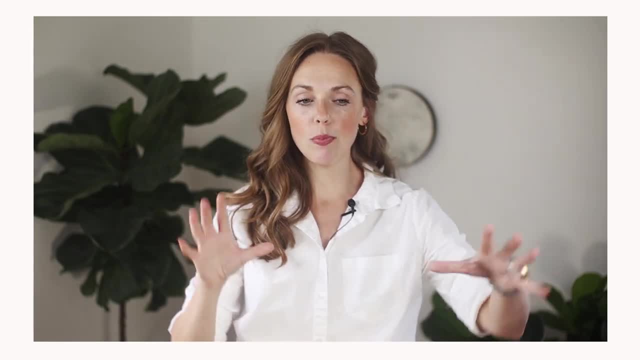 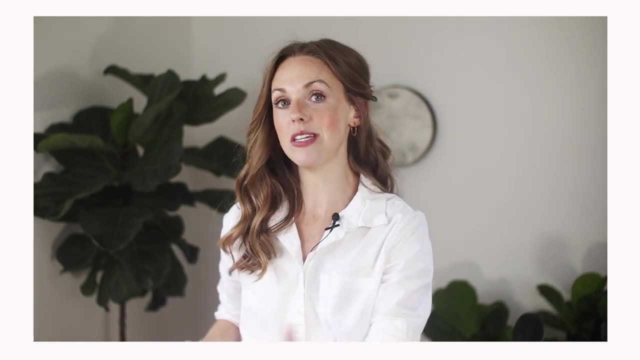 Now all of that seems like a lot, and it is, but when you put it all together it takes like three or four minutes- not very long at all because we're moving through each of these sections very, very quickly. It's like 10 seconds at each kind of stop in our warmup routine. 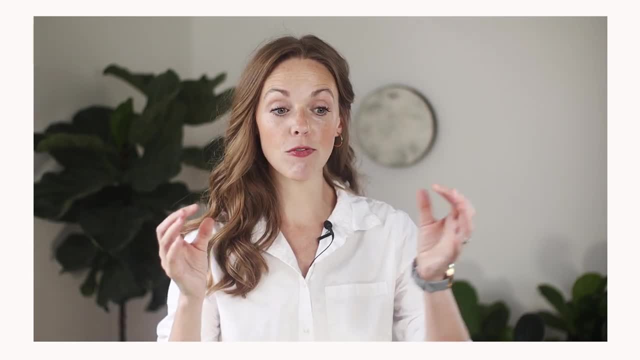 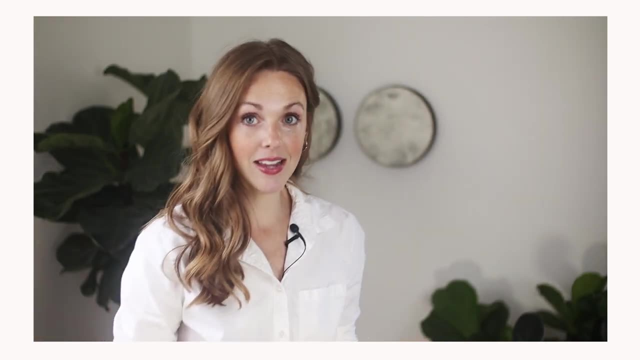 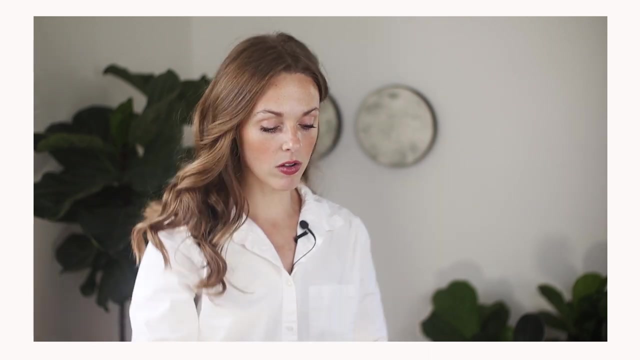 So let's talk about, in the first weeks of school, getting students from outside the room to inside the classroom. We'll start by greeting them outside and we're going to make our feet do a steady beat motion And then, just silently, we are looking at students' feet And when we see people who are doing what we are doing with, 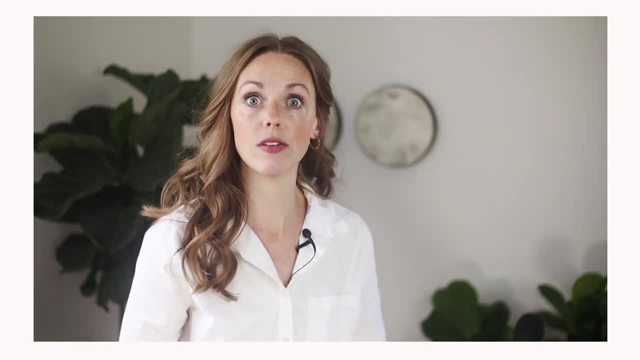 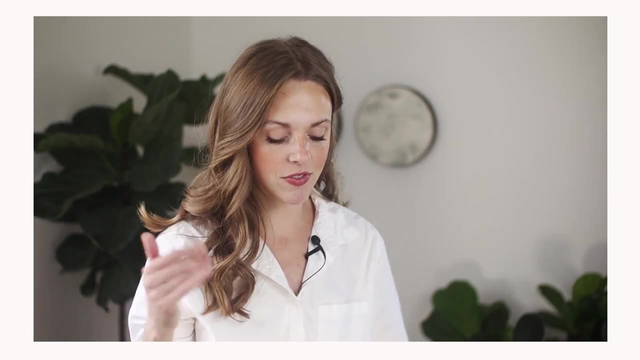 our feet. we go like it's something very interesting, very exciting, And I can see all of these people whose feet are matching mine. They hit the ground when my feet hit the ground, That's very exciting. As few words as we can do here, as possible, that is what makes this whole warmup routine. 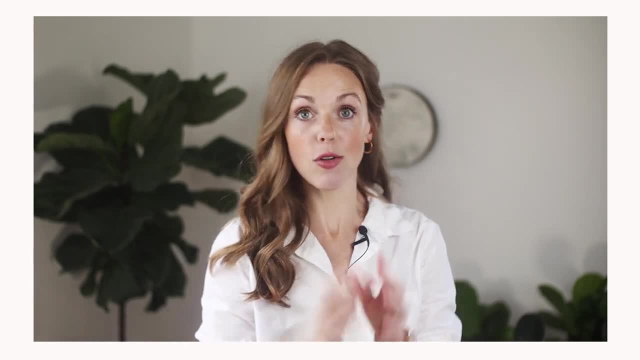 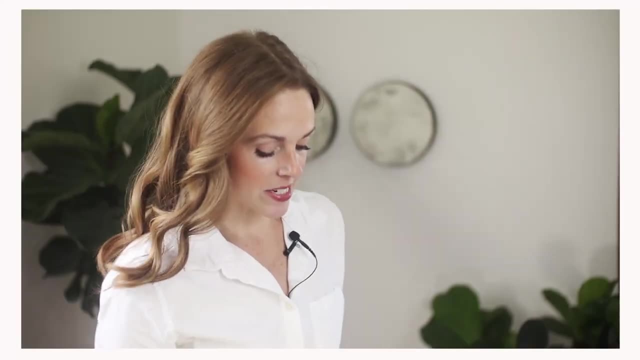 a little bit more magical, right? Okay? So let's talk about the warmup routine for the first weeks of school. All right, So we greet students outside, We've done our steady beat in our feet thing, And then we're going to say please stay in a line when we walk into the room. 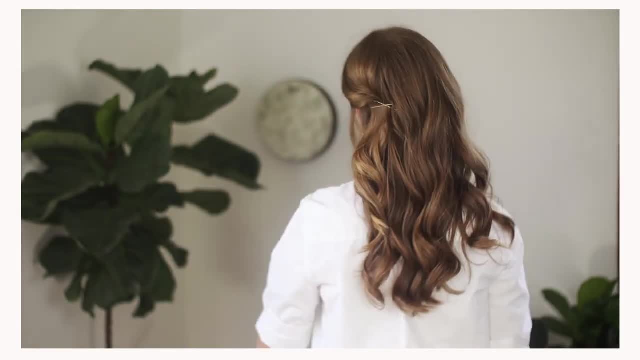 and listen to our song: Feeling fine, it's music time. Stay in a line. stay in a line. Feeling fine, it's music time. Stay in a line. stay in a line. Feeling fine, it's music time. Stay in a line. stay in a line. 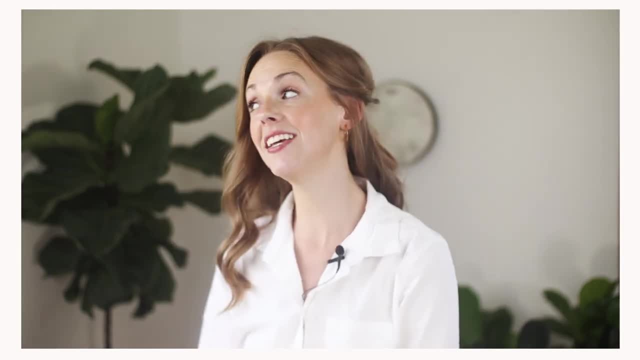 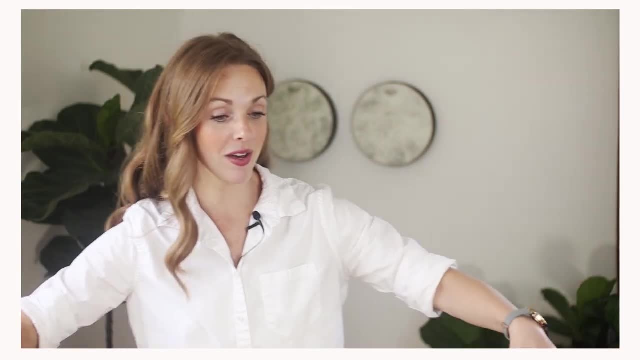 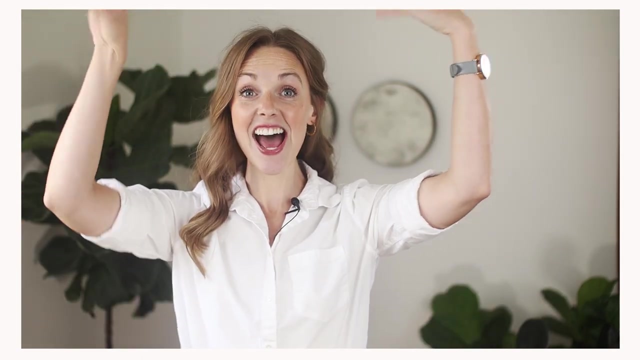 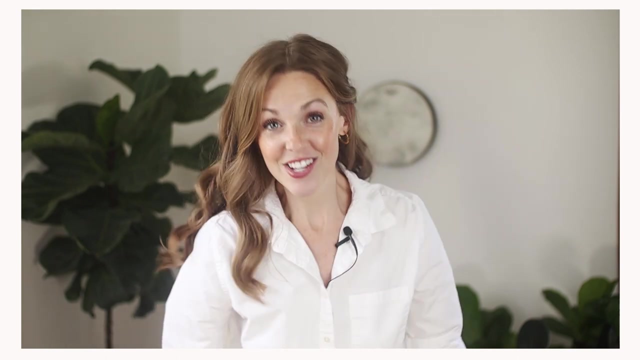 Feeling fine, it's music time. Stay in a windy line. Feeling fine, it's music time. Eventually, we lead the class in a circle. Feeling fine, it's music time. We're standing in a circle, Shake our hands high, We shake our hands low, Turn around and here we go, Feeling. 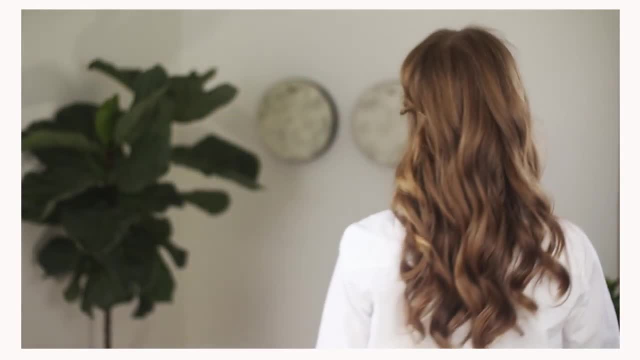 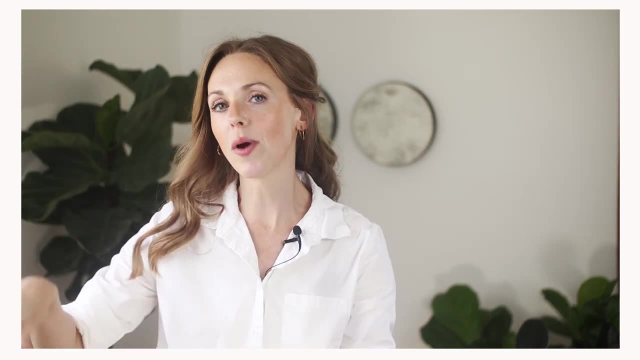 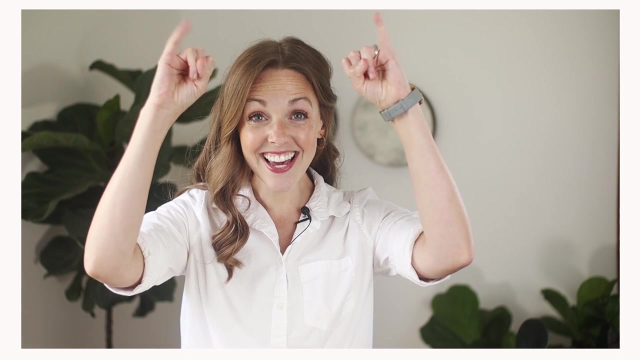 fine, it's music time. Stay in a winding line- Feeling fine, it's music time. Stay in a light in a line. stay in a line, feeling fine, it's music time. stay in a windy line. so there we're just going to walk around in the circle formation that we've led students into. we wiggle our pinkies high. 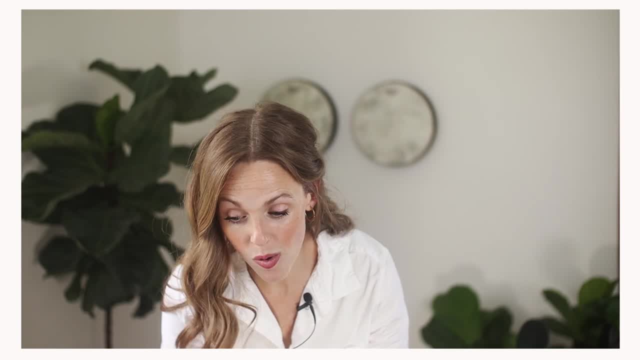 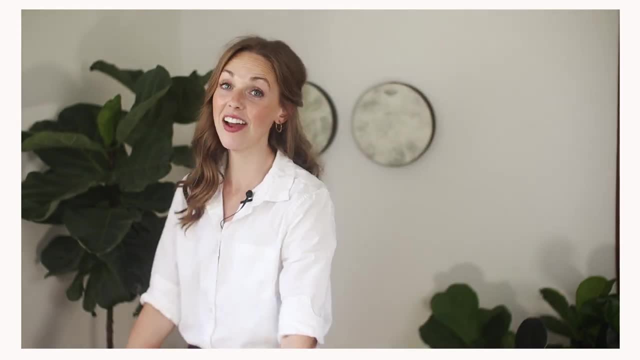 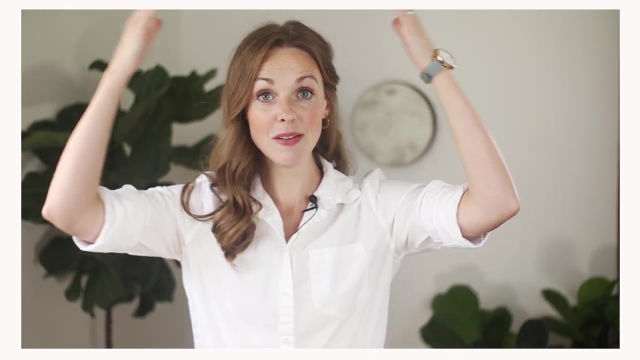 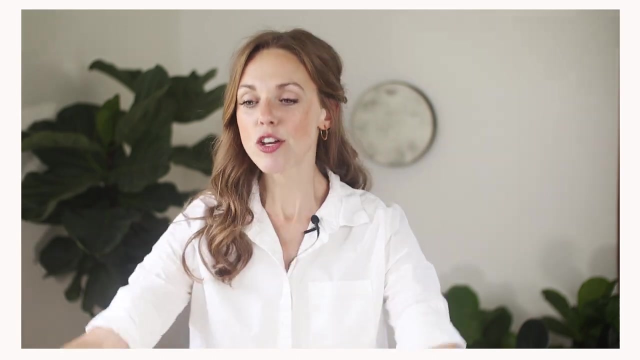 we wiggle our pinkies low, turn around and here we go, feeling fine, it's music time. stay in a line. stay in a line, feeling fine, it's music time. stay in a windy line: feeling fine, it's music time. stay in a line. stay in a line, feeling fine, it's music time stay in a windy line. so, moving into some, 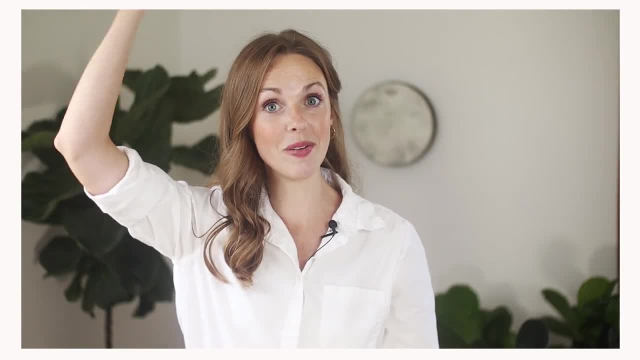 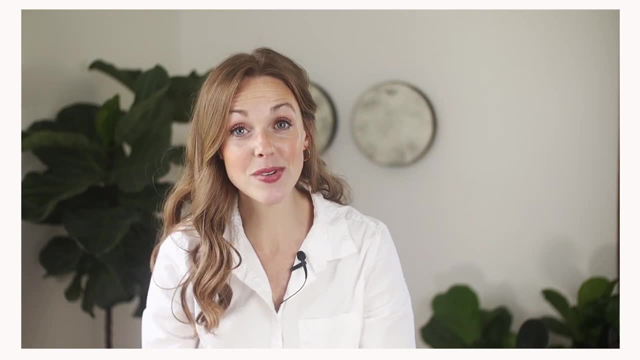 steady beat motions and we don't tell students that that's what we're doing. we just start to do it feeling fine, it's music time. stay in a line. stay in a line, feeling fine, it's music time. stay in a windy line moving our pinkies high. 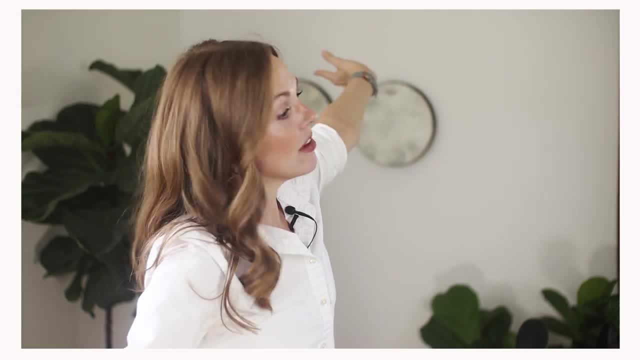 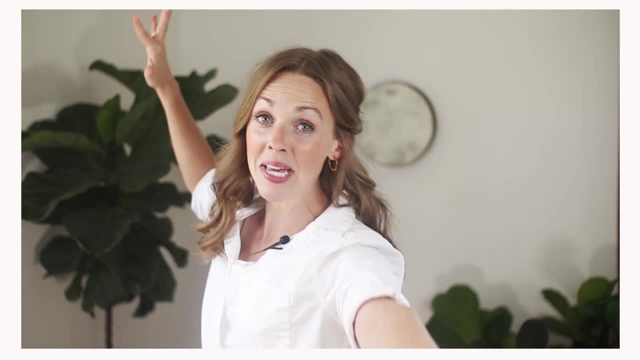 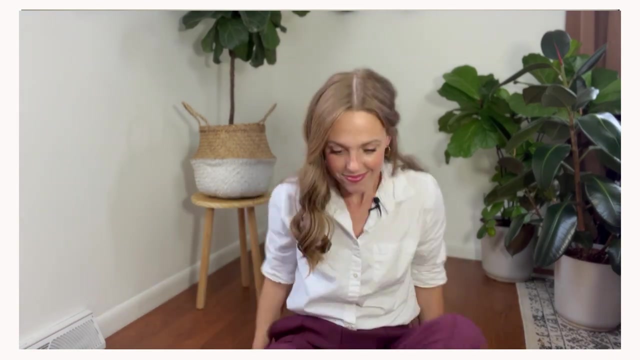 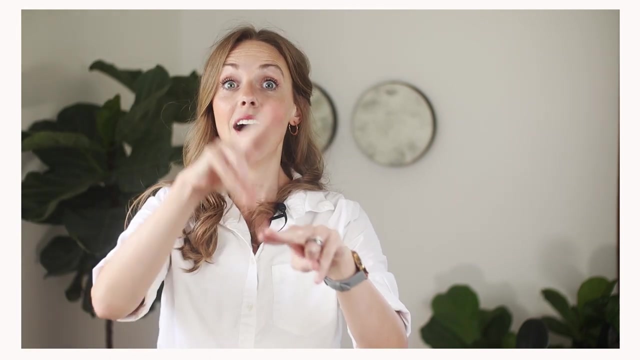 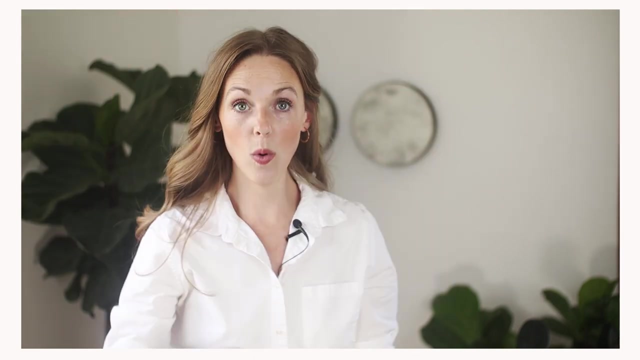 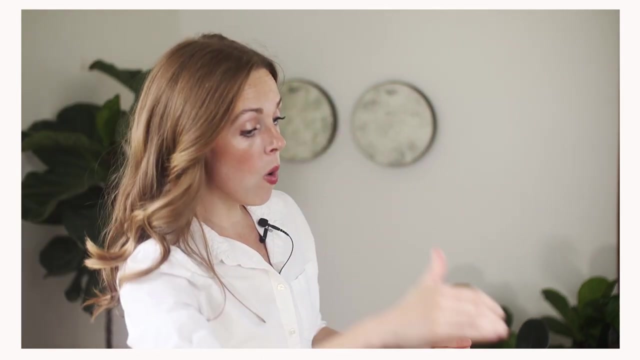 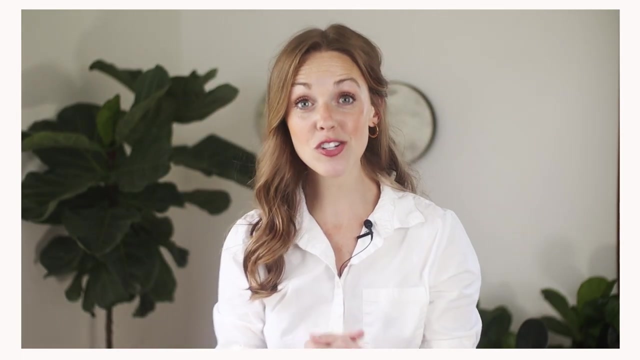 leading through some stretches and we can give verbal um prompts to students like: oh, i see your body looks just like mine. oh, i see that your hands are doing what my hands are doing: some motions for sit and stand, hello, first grade. or hello second grade. how are you today? 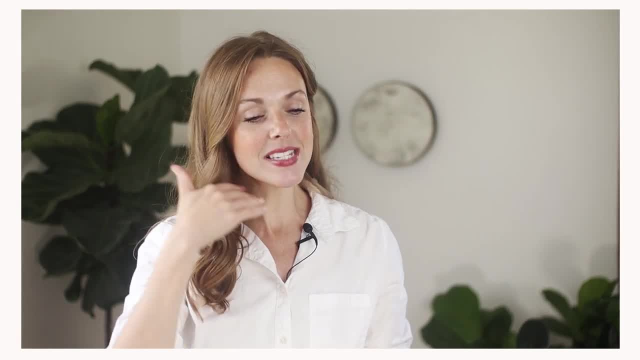 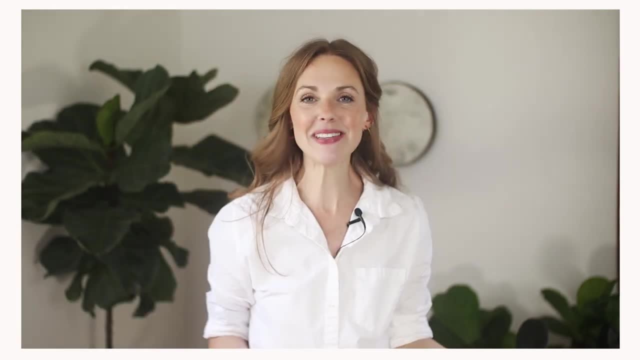 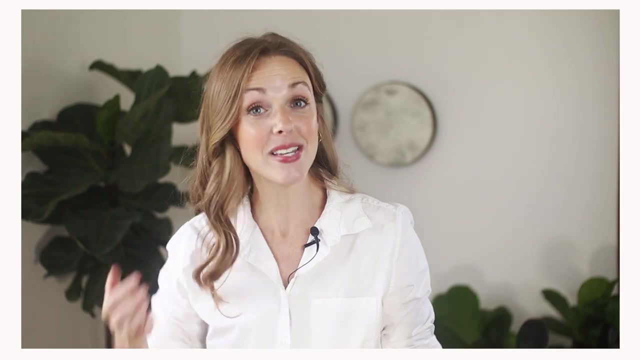 and when we sing hello first grade, if we get back hello first grade, we're just going to say my name is not first grade, my name is mrs victoria. so when i sing hello first grade, you may respond: hello, mrs victoria. let's try it. hello first grade. 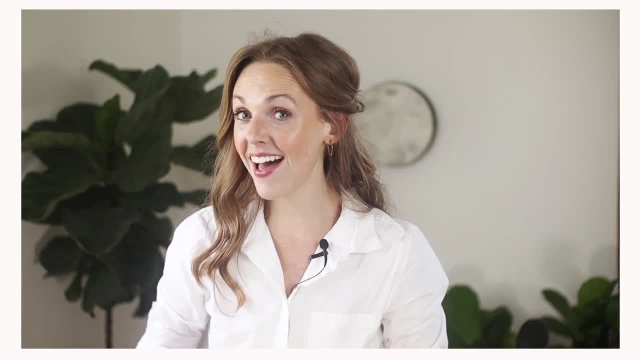 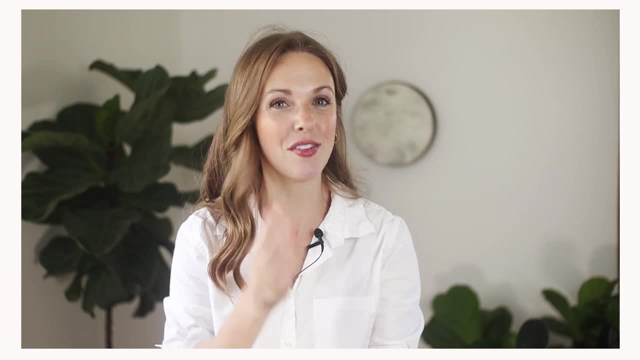 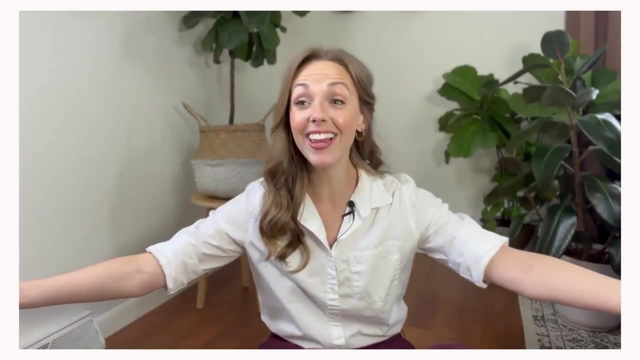 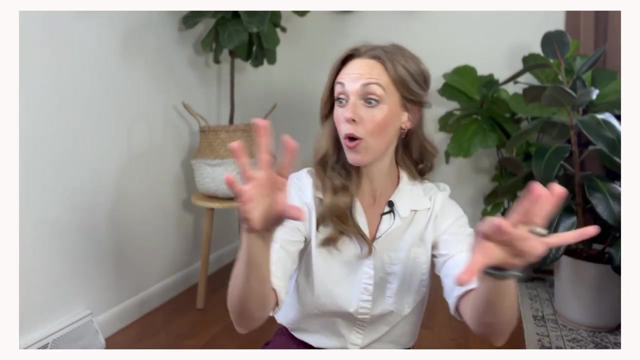 how are you today? and whatever response we get from our first graders, second graders, great. it's the first day of school, the first two classes, and we're going to build from that. i'm so glad you're here. i'm so glad you're here. i'll wiggle my fingers to say hello, i'm so glad. 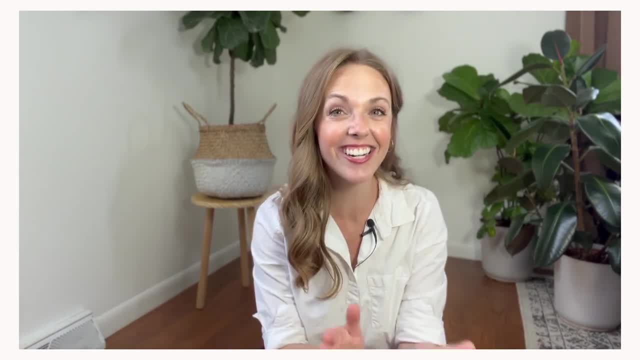 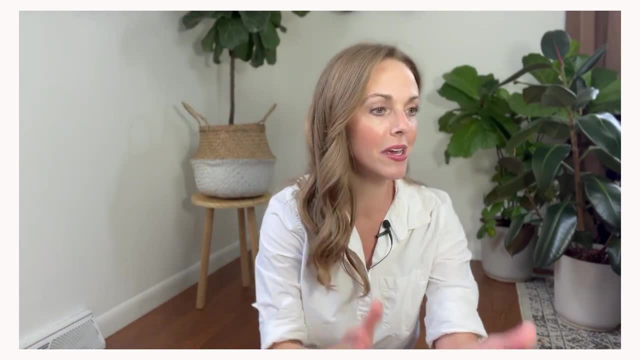 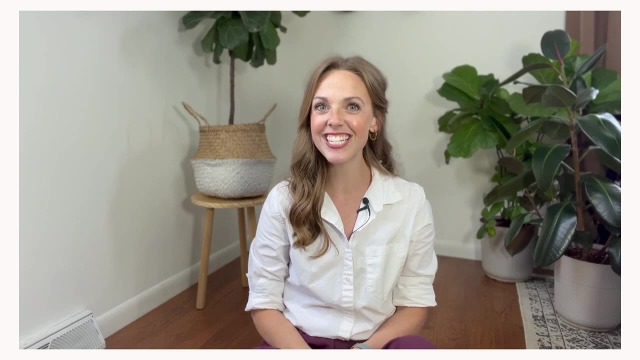 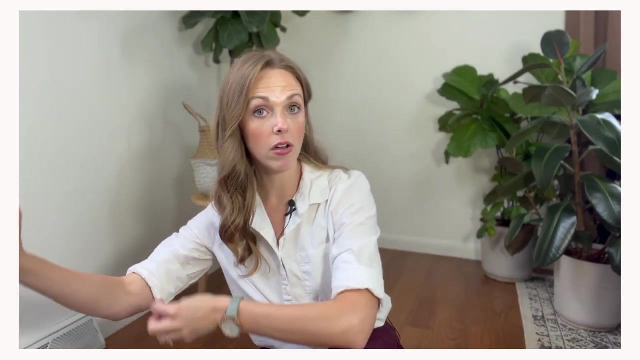 you're here. i'm so glad you're here. i'm so glad you're here. i'll wave my hand to say hello, i'm so glad you're here. i'm so glad you're here. you get the idea. i'm so glad you're here. i'll wiggle my toes to say hello, i'm so glad you're here. as we continue with this song. 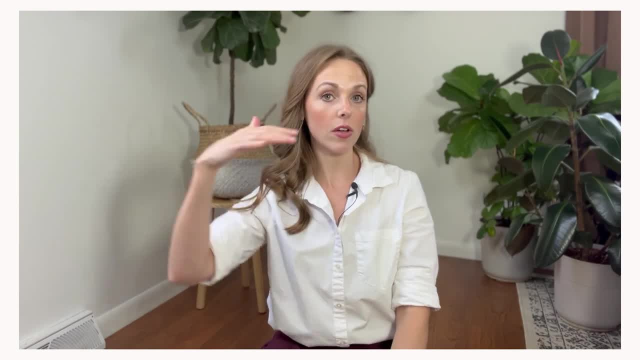 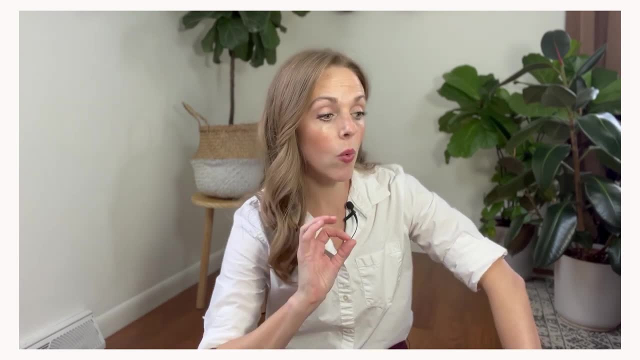 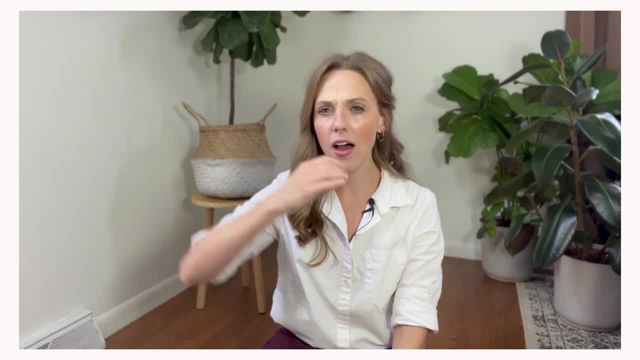 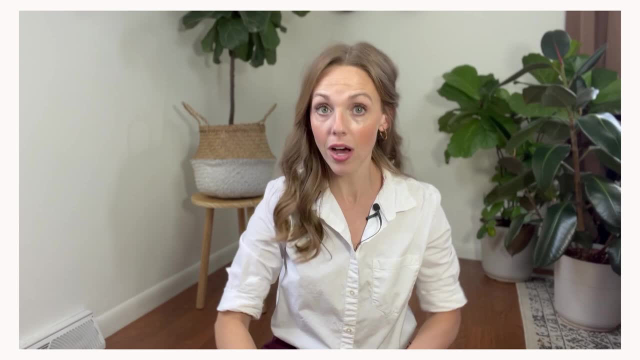 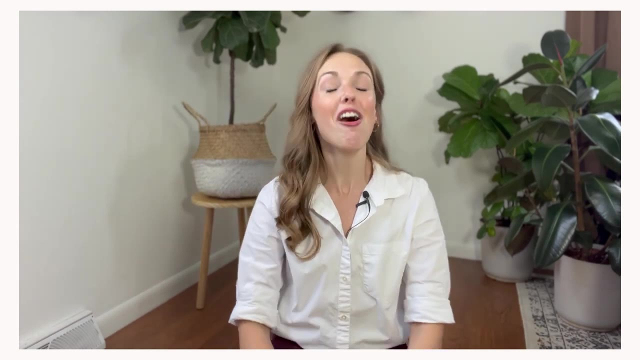 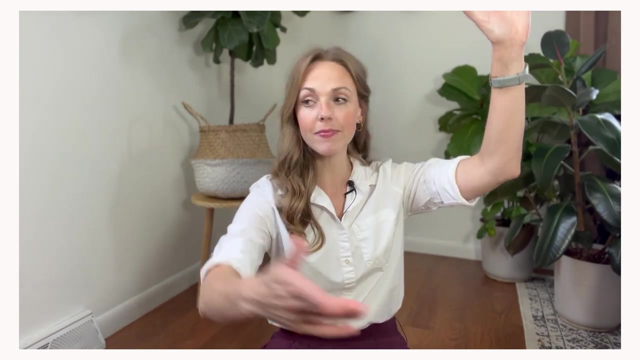 you're here. i'll just put my hand in the air silently to ask students what they think we should do, and someone's gonna say i'll nod my head: great idea, i'm so glad you're here. i'm so glad you're here, i'll nod my head to say hello, i'm so glad you're here. someone's gonna say, um, i will smile. 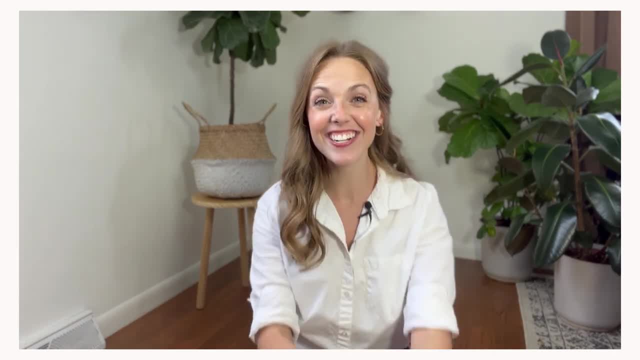 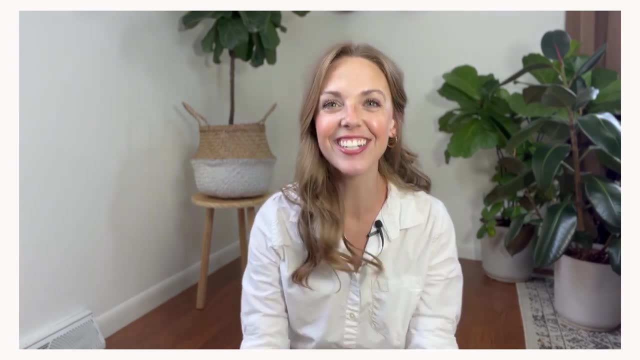 with my teeth. great idea, i'm so glad you're here. i'm so glad you're here. i'll smile with my teeth to say hello, i'm so glad you're here. so very, very simple, um kind of introduction to this song, and this is one that 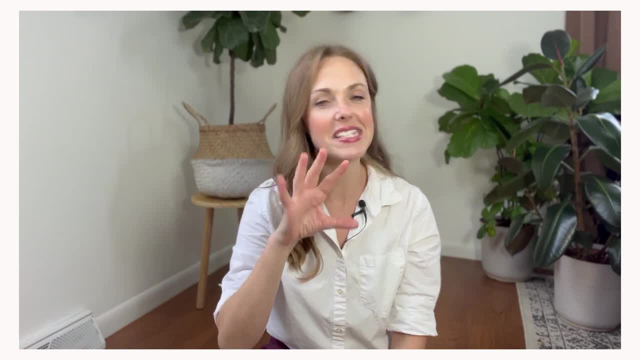 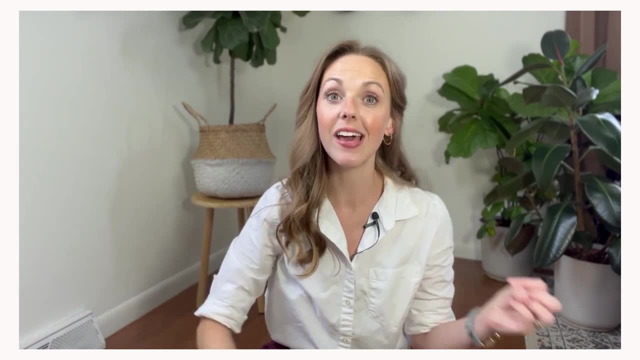 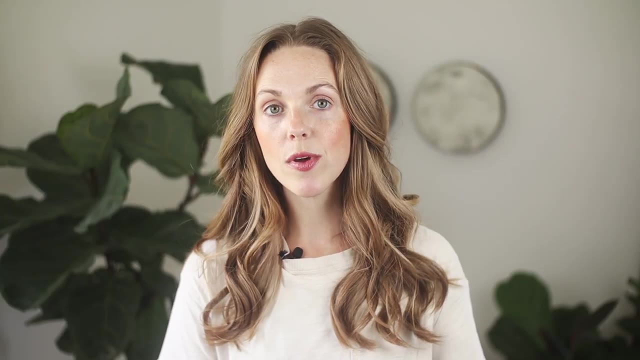 we will have several layers on top of, especially for, like a second grade ish area, um, but for the first several weeks of school, just asking students how they want to say hello to each other- beautiful way to start class: with a welcome song. you can also get to know the other members of our ensemble and i mentioned that our interactions are. 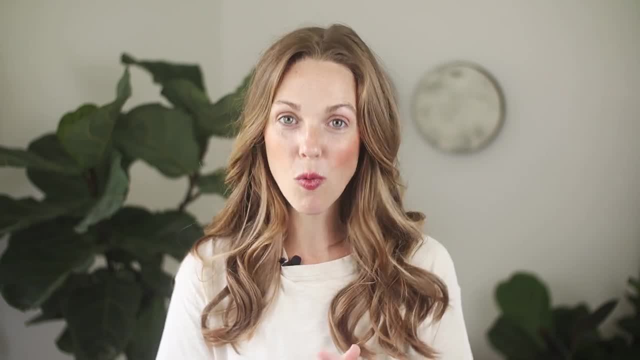 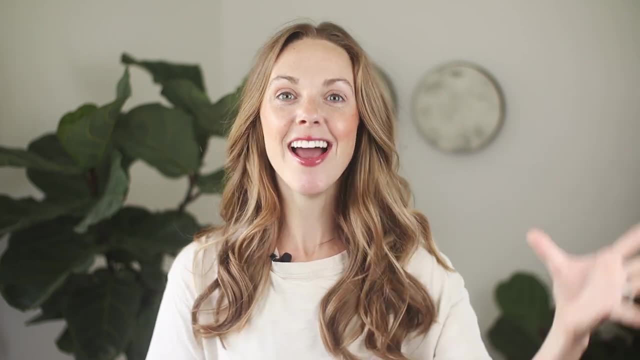 going to take place within a musical ensemble, so getting to know the other members of our ensemble is super important, both for us and for the other student musicians in the room. so, uh, we just came from lower elementary. now let's do a getting to know you activity for upper elementary and that. 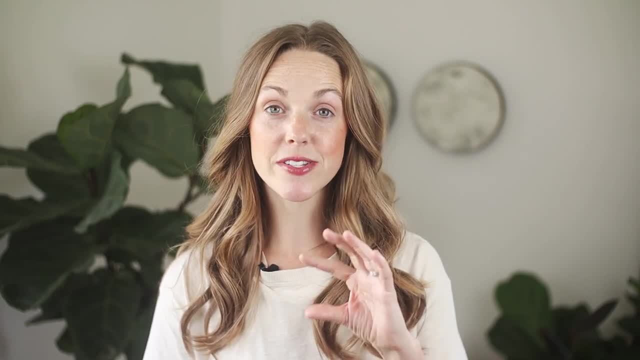 is going to transition into a name game now. i mentioned some slides in this video and and those editable slides are inside the planning binder. but this could just as easily be used to learn about the planning binder. but this could just as easily be used to learn about the planning binder, because weね. 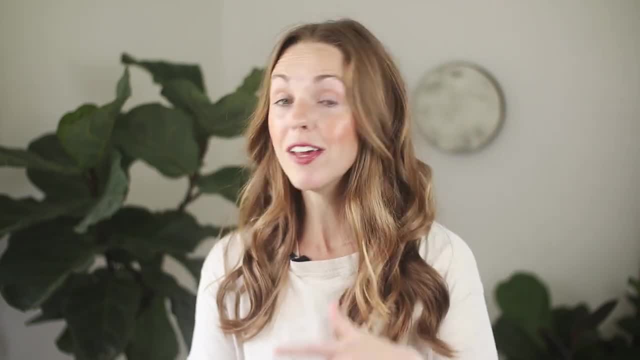 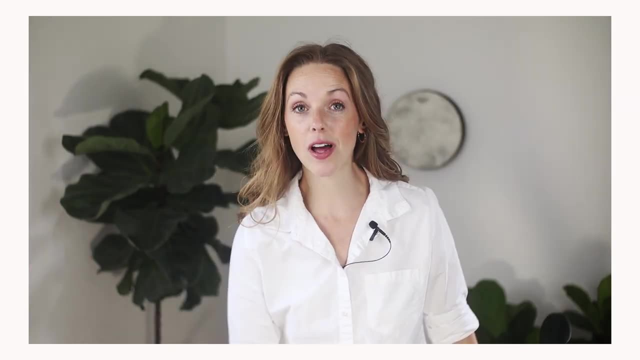 be just a list of questions that you write on the whiteboard, right. So here is Hey Lolly, and Up the Ladder, Down the Ladder. Will you copy my motions? We're all standing in a circle. I'm starting with my right leg, Make sure you know. 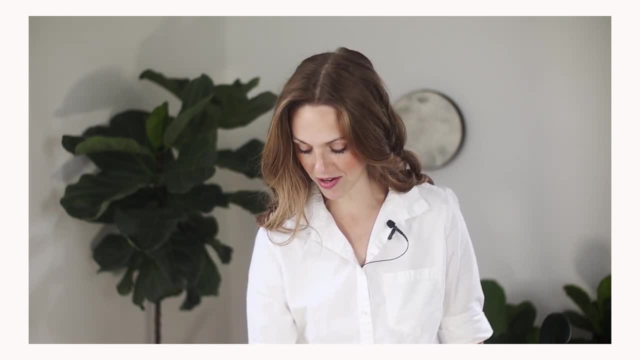 which one is your right foot and which one is your left foot. Point to your right foot. Make sure it's the same as all of your neighbor's right feet Should be opposite from mine if you're facing me. People on the sides have kind. 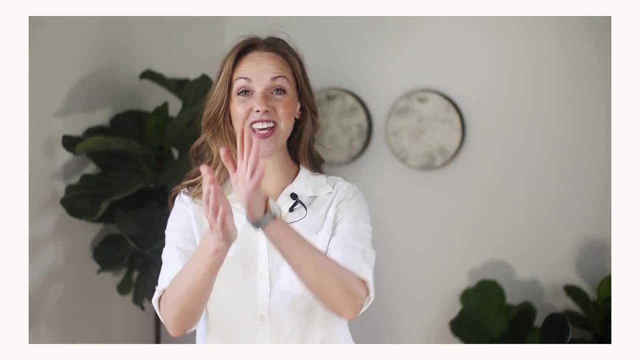 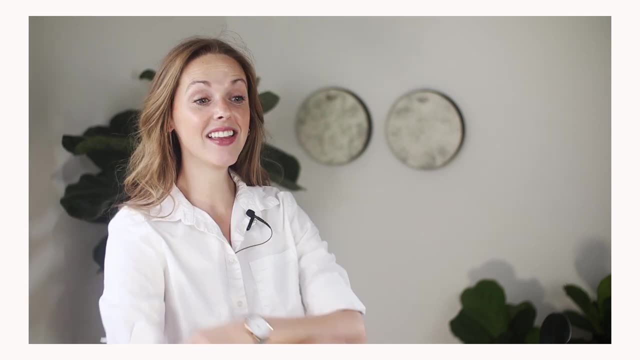 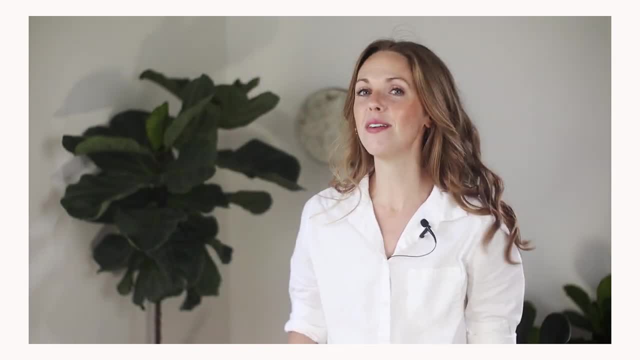 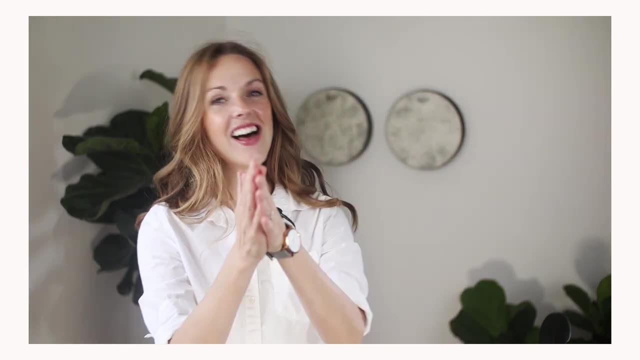 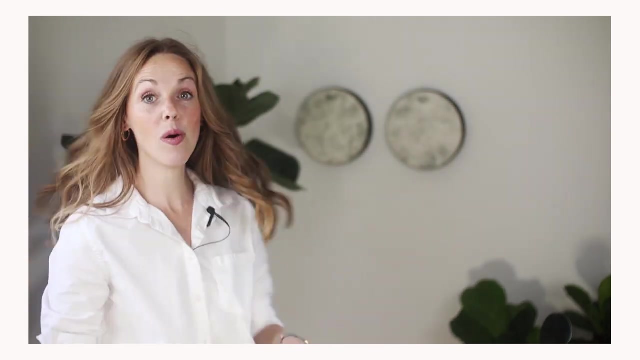 Interesting. what do you notice? Hold your answer in your head Doing the same thing again. You're not singing, just copying my motions. Hey, Lolly, Lolly, Lolly, searching you again, you're not singing, just copy my motions. hey, lo, What do you notice? Turn and talk, And then we'll give our signal for students to stop talking. 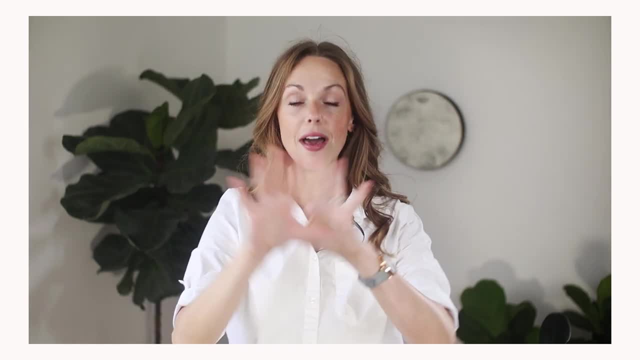 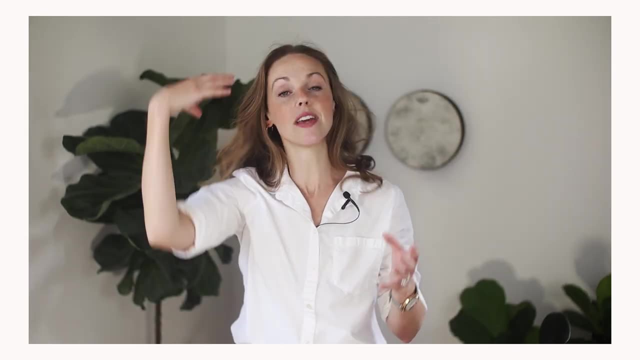 whether that's a hand in the air showing them a quiet thumbs up If you have a chime, whatever it is that you have already established in your procedures. this is our time that we are practicing And students might have all sorts of things that we notice. My next question for you: 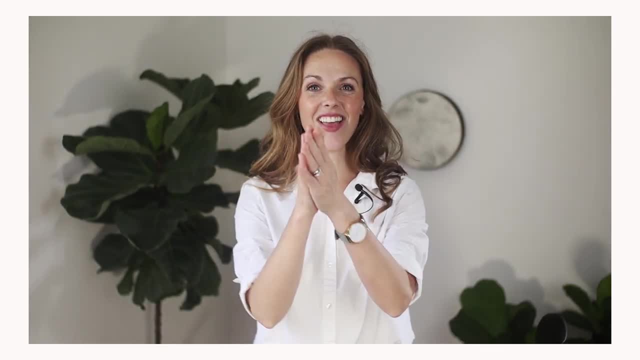 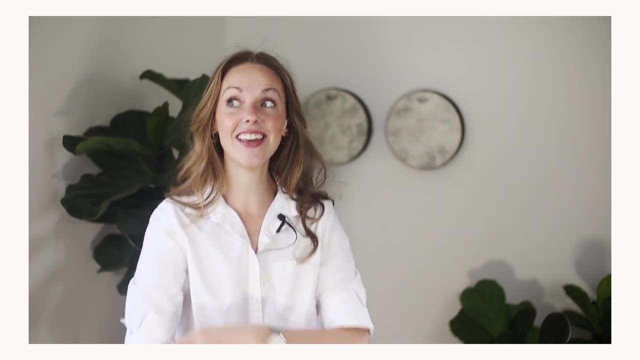 is there a pattern? Here you listen: Hey, lolly, lolly lolly, Hey, lolly lolly lo, Hey, lolly, lolly lolly, Hey, lolly, lolly lo Great. After a while we've done this several- 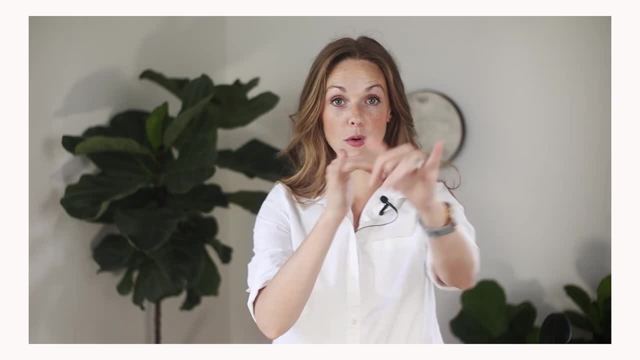 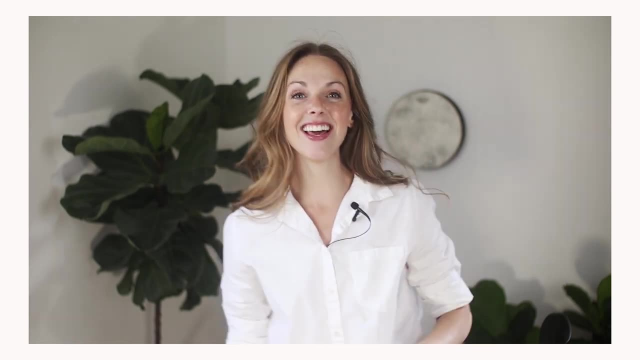 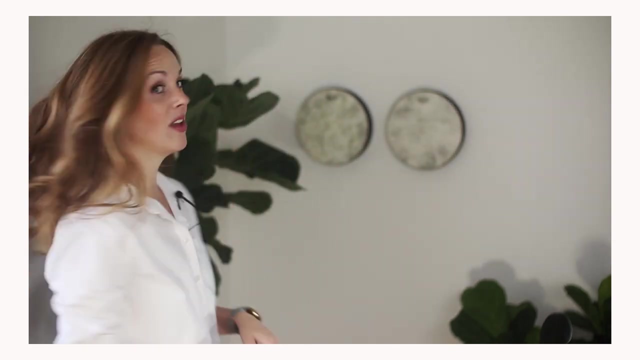 different times and we can invite students to sing as they are doing our motion. So let's do it together. Just teacher talk. Starting with our right foot, Here we go. Hey, lolly, lolly, lolly, Hey, lolly, lolly lo, Hey, lolly, lolly, lolly. Hey, lolly, lolly lo. Beautiful When I 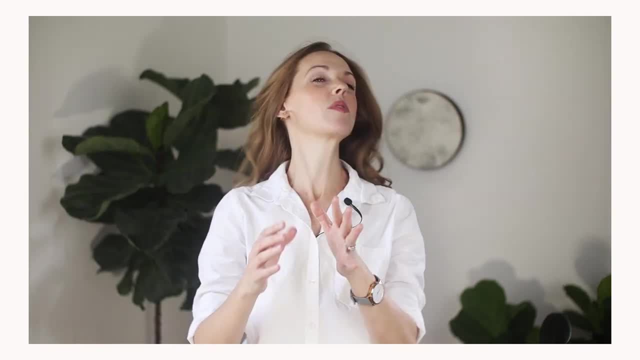 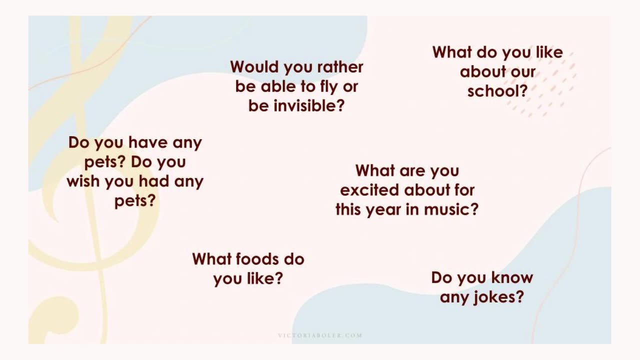 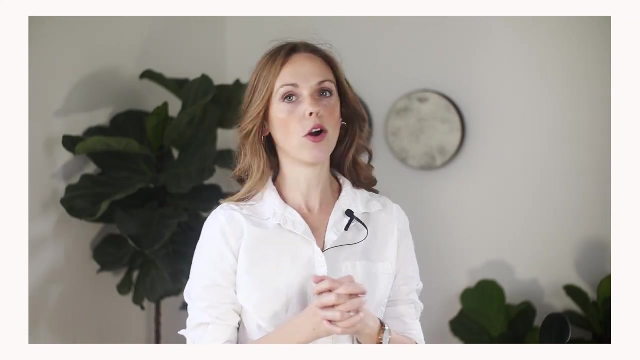 say go, third grade, fourth grade, fifth grade, whatever grade we're using this with. When I say go, I would like you to find a partner and you may answer any of the questions on the board that you like. When I say what Go? What if I say green beans Don't go? What if I say a go-gurt Don't? 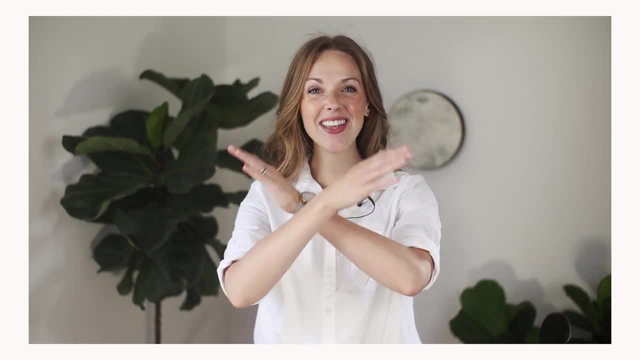 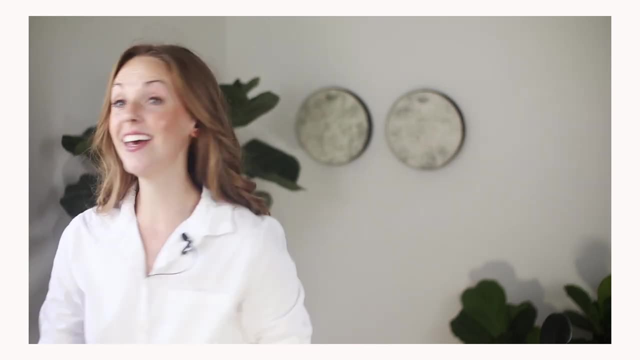 go Here. we sing to the right: Hey lolly lolly lolly, Hey lolly lolly lo, Hey lolly lolly lolly, Hey lolly lolly lo Go. 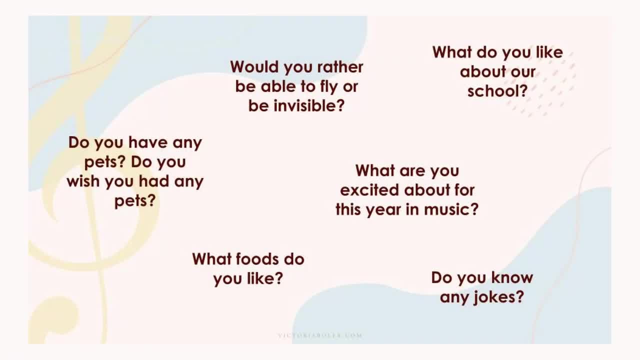 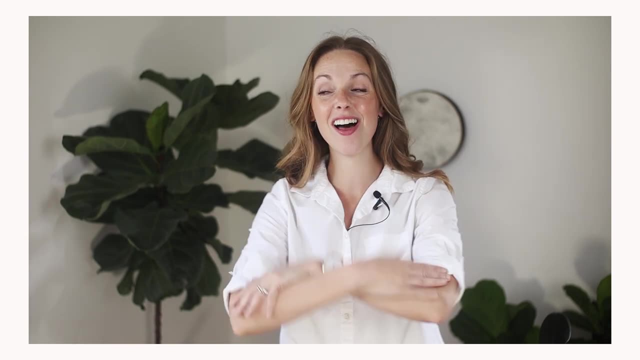 These questions on the board are editable, so you can change them up for whatever questions you would like students to work with on their own, And we'll give a five, four, three. back to the circle. Here we go, And hey, lolly, lolly, lolly, Hey, lolly, lolly, lo Hey. 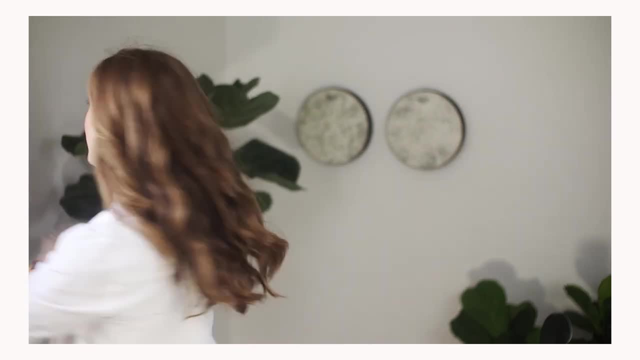 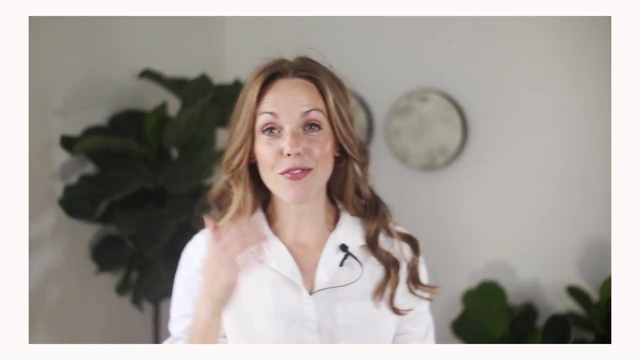 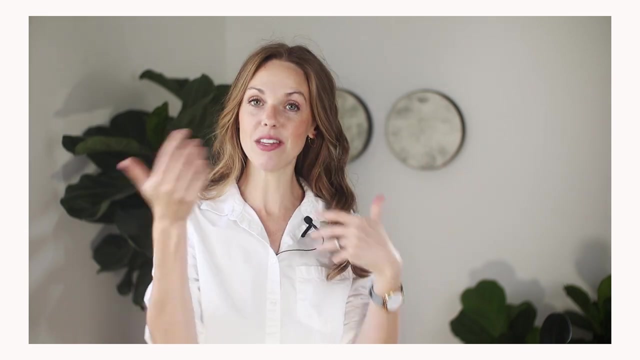 lolly lolly lolly. Hey, lolly lolly lo, Freeze, Don't move. Find someone different, Go. So we go through this several different times. Students need to find a different partner each time. They can answer the same question each time if they want, or they could pick a different. 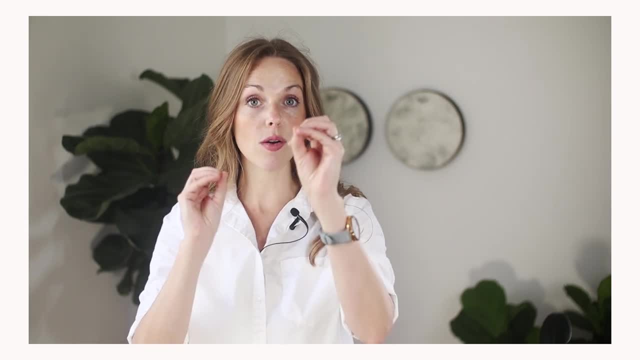 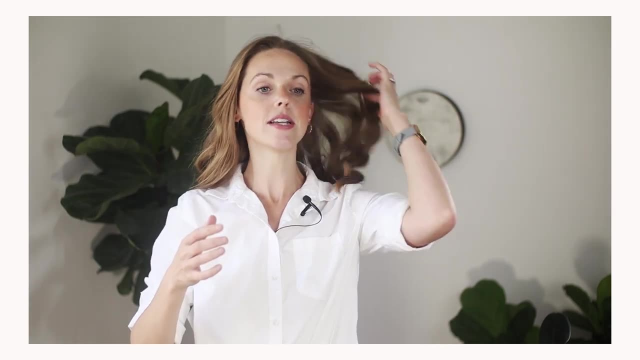 question each time, if they want, When students are ready. maybe it's this class, very likely it will be in the second class. We can move to a double circle, So a nice way to do this is go through the activity in this next class. Hey, lolly, lolly lo, Find a partner Now when you. 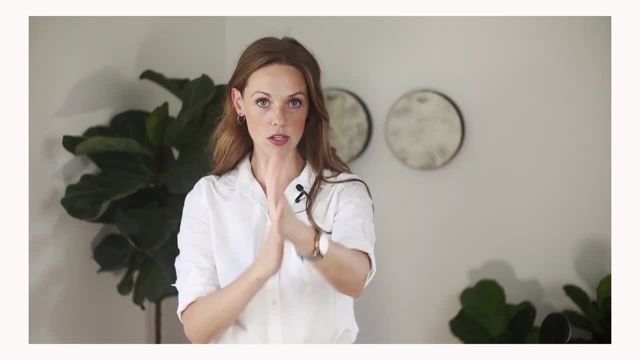 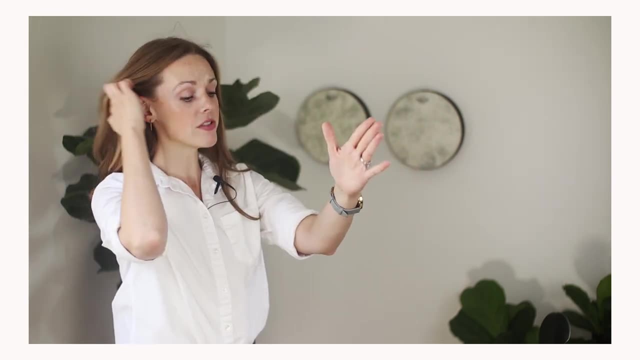 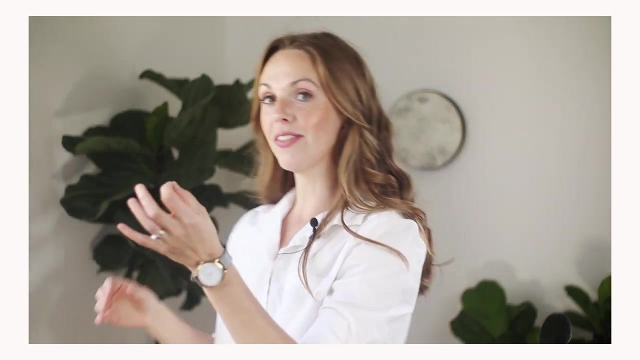 have an outside circle and your partner is facing you. so if you have an outside circle with a partner facing you, now we have an outside circle and an inside circle. So let's imagine that I'm on the outside circle. I'm going to take a step to my right. Hey, lolly, lolly, lolly If I'm. 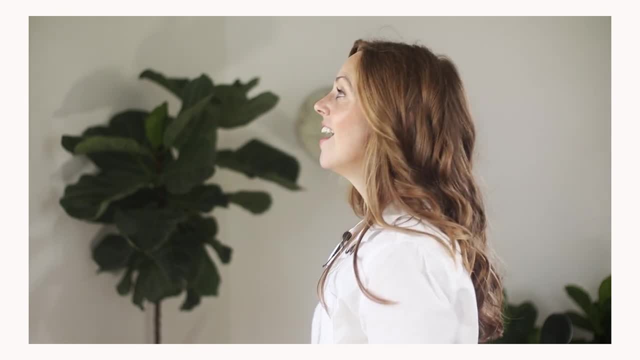 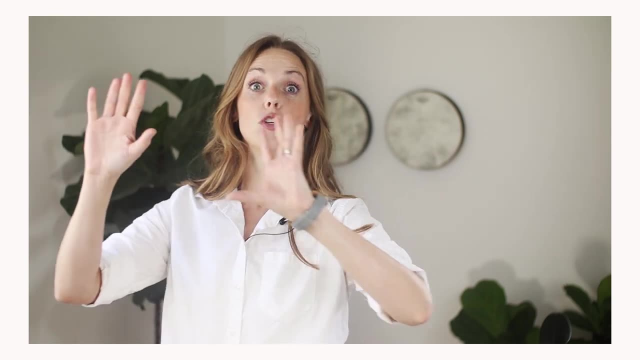 on the inside circle. what am I going to do? I will also take a step to my right. Hey, lolly, lolly, lolly. And what happens is, as I move to the right and you move to your right, all of a sudden, 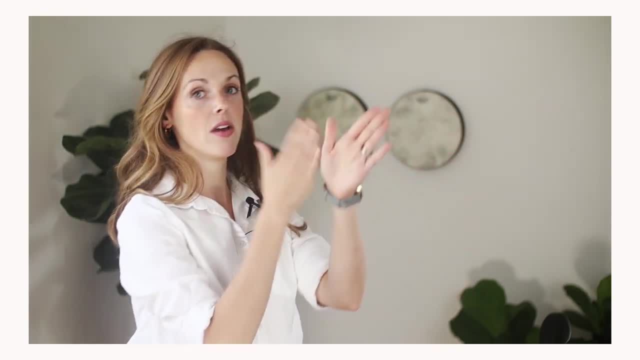 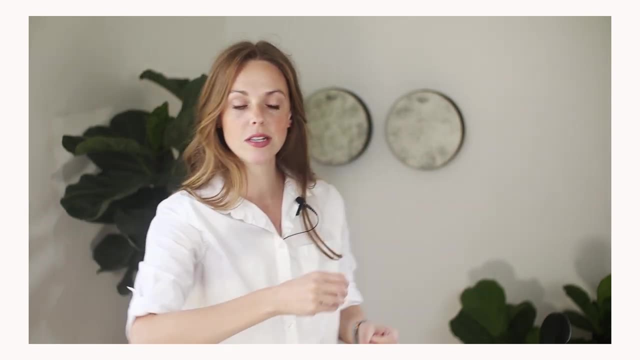 we have switched partners, So now every time we take a step to the right, we'll be facing a different partner. We can keep this Hey, lolly, lolly, lolly Or, if you want to level it up again, it just depends on how much experience students have with this rhythmic agency over. 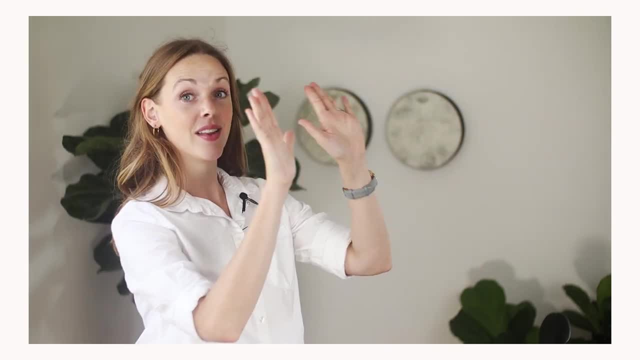 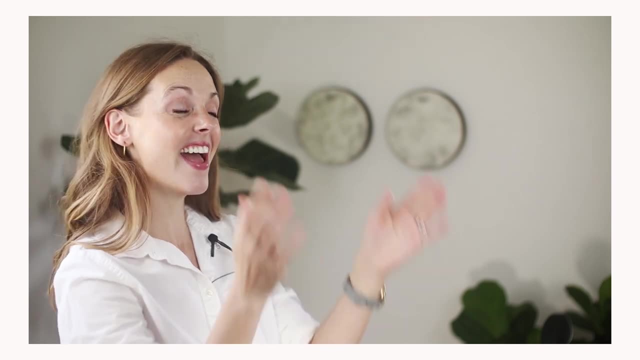 their bodies. We can change it to: hey lolly lolly lolly, New partner. Hey lolly lolly lo, New partner. Hey lolly lolly lolly, Last partner. Hey lolly lolly lo. 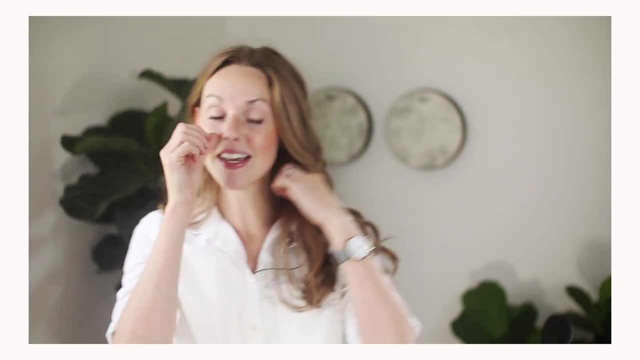 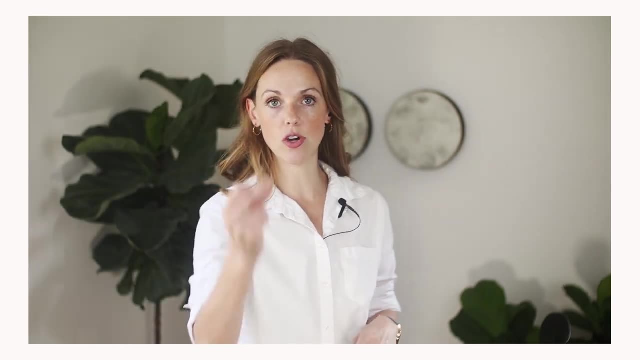 Excuse me. Hey, lolly, lolly, lo Keep the spin at the end, But now I am paired with someone in this double circle dance, So we are not going to do. the teacher says: go and you find a new partner. 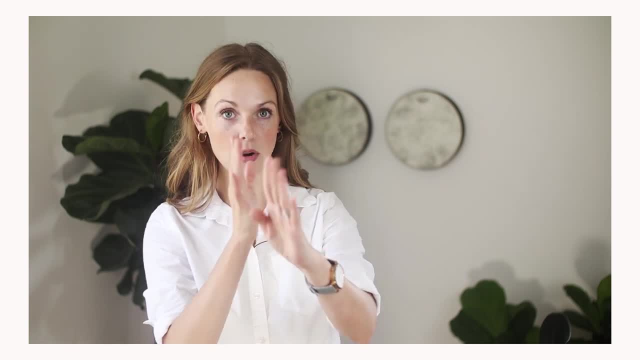 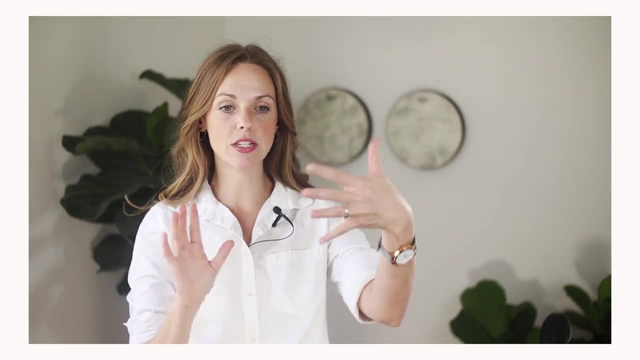 Now, whoever you land with at the end, that is the person that you will have this discussion with, with the questions on the board, And if we do this several different times, students will have the opportunity to interact with number one- everyone in the circle- because we switch partners. 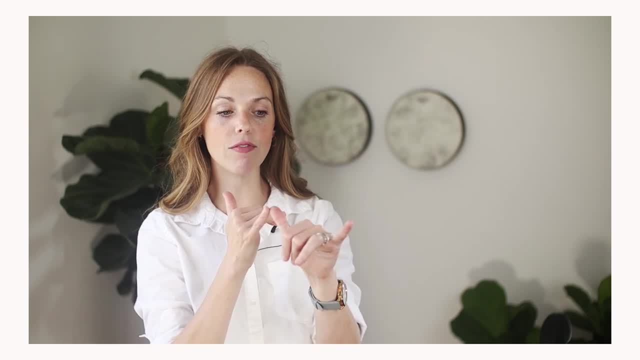 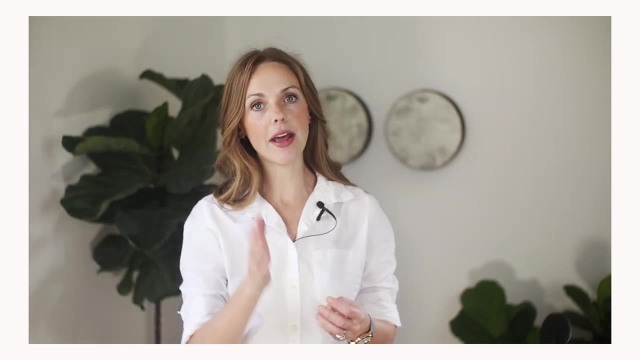 and we clap, Or number two, we will also be able to interact with the other students. So now we're going to also have the opportunity to have some of these conversations, with these getting to know you questions, with other people in the circle who we might not have chosen otherwise, And 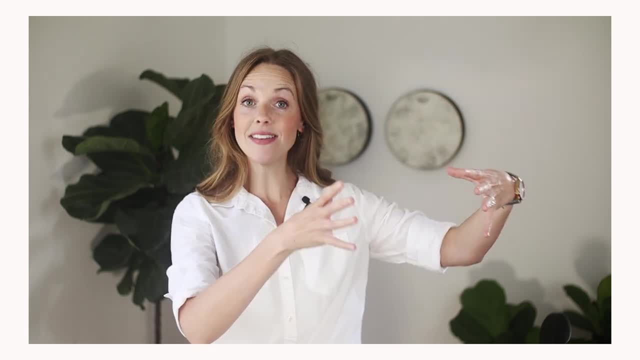 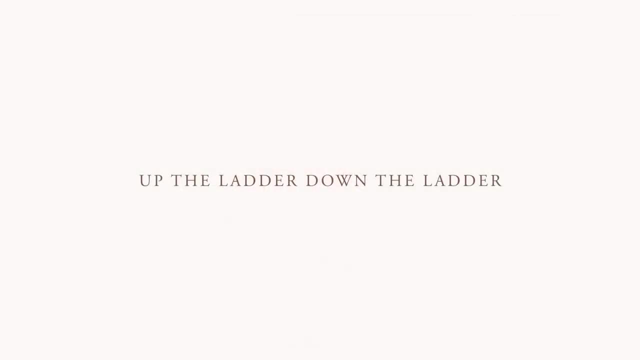 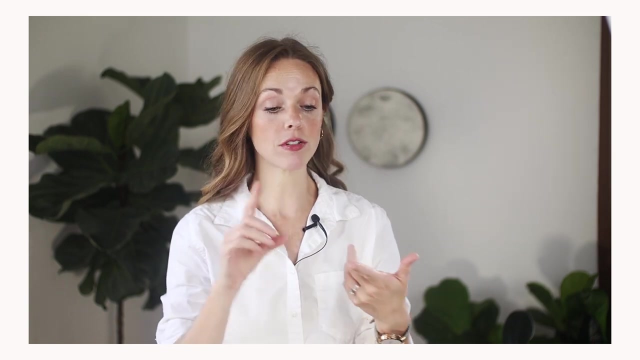 that's the value of moving from a first class: students choose their partner. Second class, the mixer kind of chooses the partners for us, Wrapping up our activity from the getting to know you circle dance that we were doing at whatever, with whatever song we were using and at whatever. 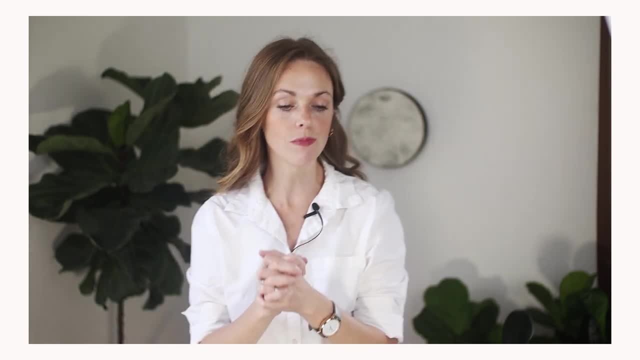 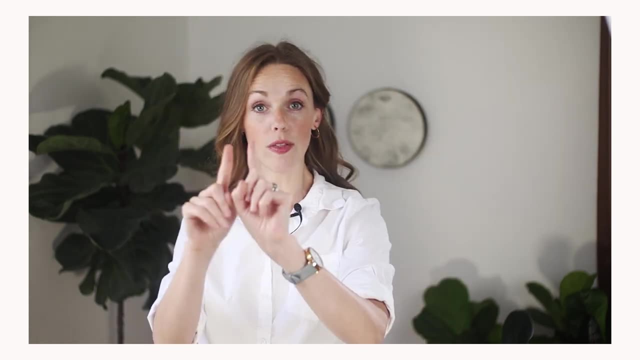 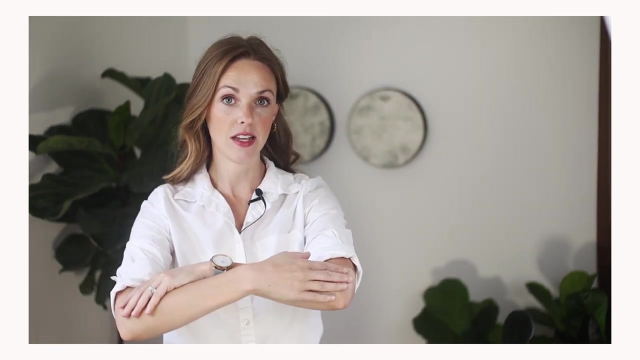 level, whether that is a single circle or the double circle. As we wrap that up, our last question to students is going to be: instead of looking at the board, can you, with your partner, decide how many steady beats are in our pattern? Students will decide four steady beats, Can you? 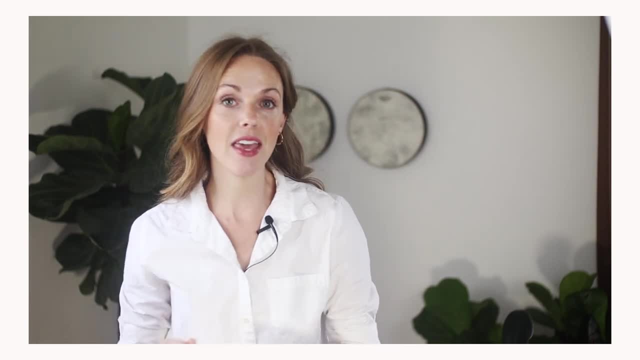 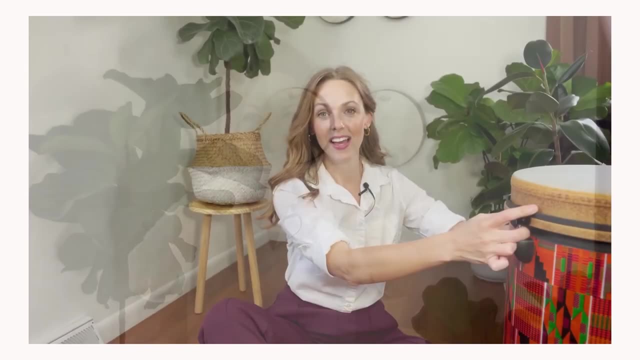 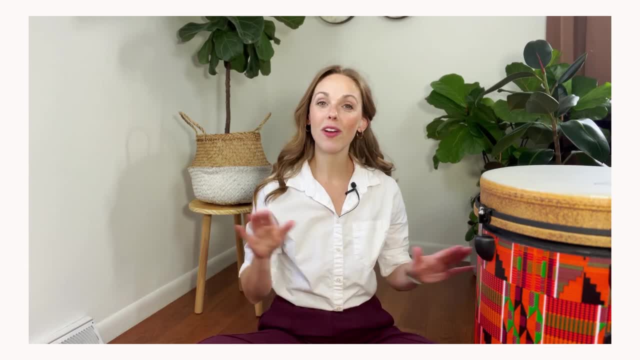 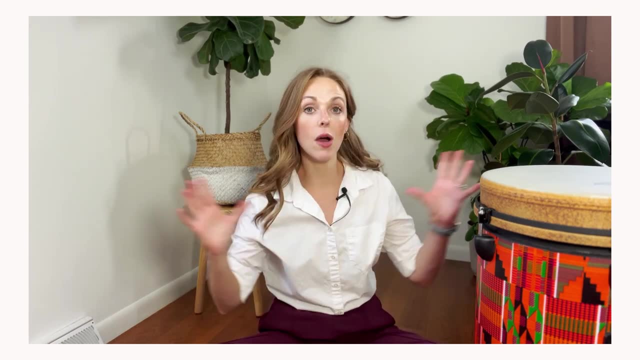 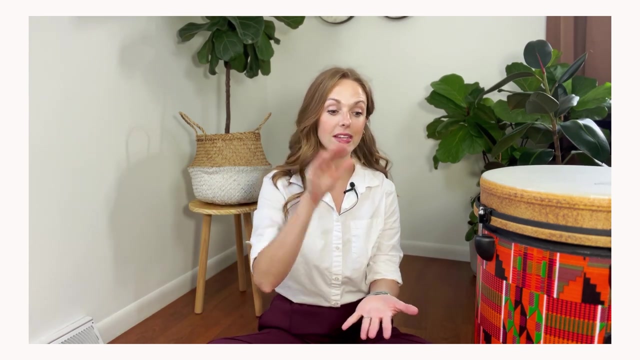 two, three, four, two, two, three, four, three, two, three, four, four, two, And we stop. Excellent, If you and your partner are not in our single circle seated, will you please move there now? So make sure everyone is seated on their spot, whether you are using sit spots. 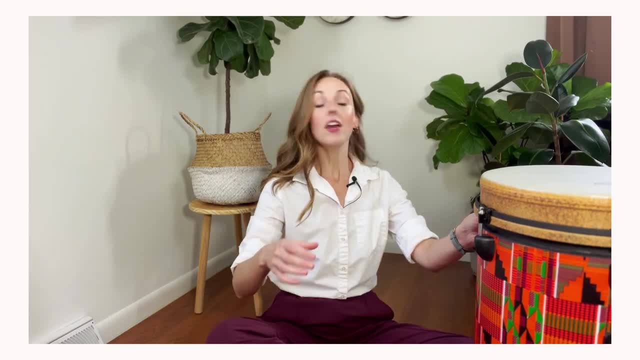 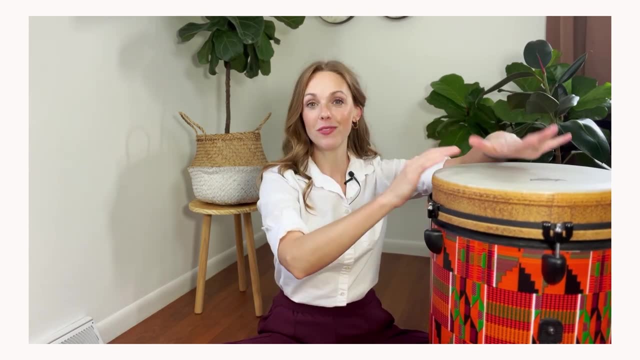 whether you have another way for students to sit on the floor in their circle. try it four times in a row. This time I'm going to try to trick you. A one, a two, a. here you go. One, two, three. 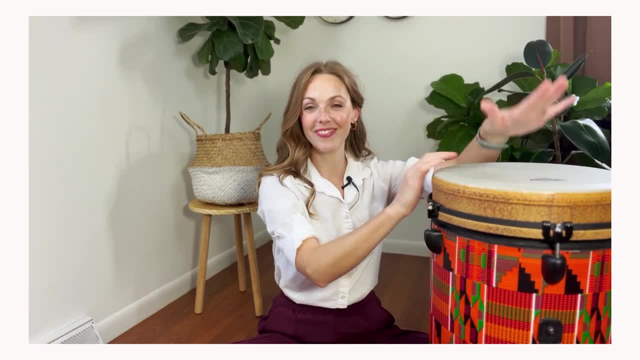 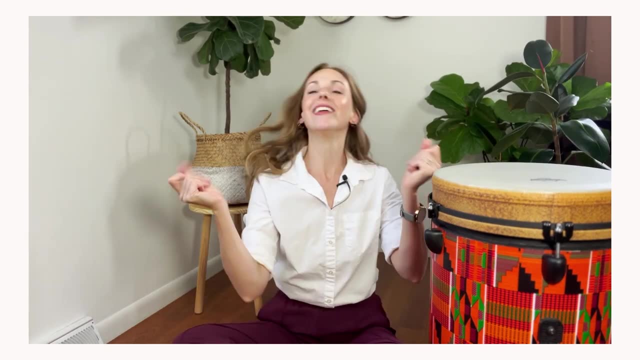 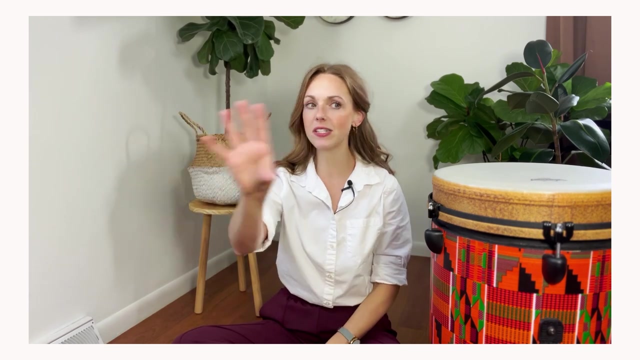 four, two, three Last time, And we stop right here. Excellent, Up the ladder, down the ladder, one by one, the ladder. Up the ladder, down the ladder, one by one, the ladder. Hmm, I'm looking around the room. I see lots of different steady beat patterns. You keep 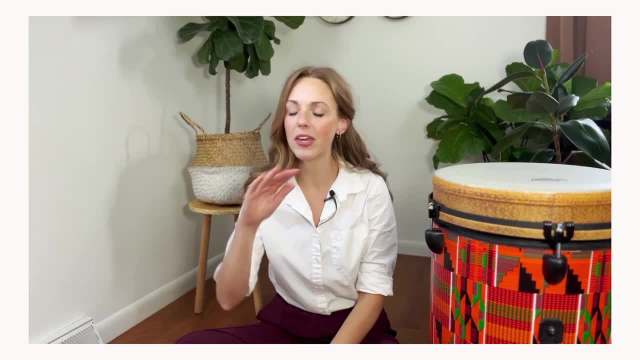 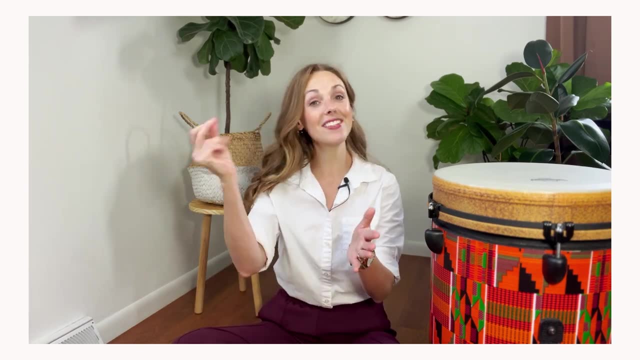 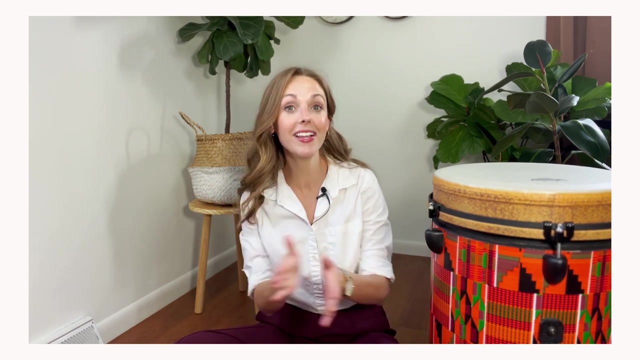 doing your steady beat pattern as you speak this with me. Very easy for students to pick up Here. go Up the ladder, down the ladder, one by one. the ladder. Up the ladder, down the ladder, one by one, the ladder. Speak it without me. A one, a two, a. here you go Up the ladder. 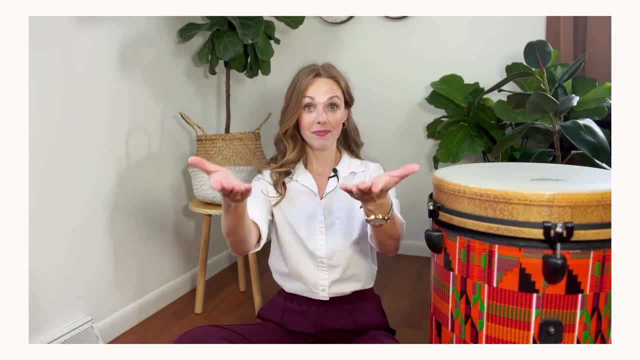 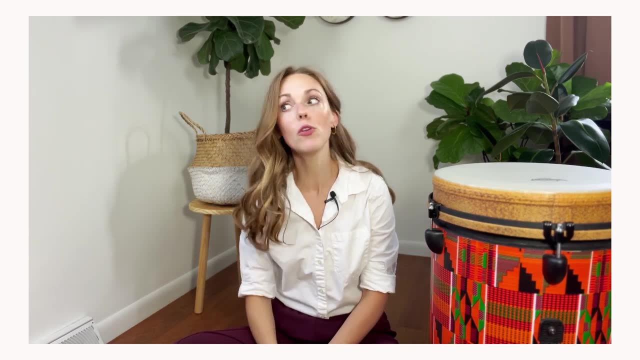 And we stop: My name's Miss Victoria And you, as students, will say back: my name is Miss Victoria And you say: no, that's not right, That's probably not your name, right, Your name is Miss Victoria is what I want you to say back. So I will say: my name is Miss Victoria, Your name is Miss Victoria. 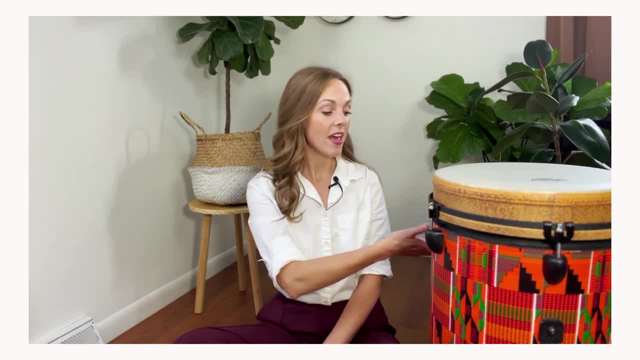 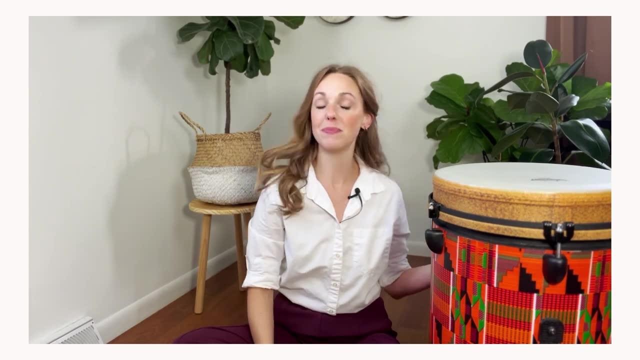 I'm going to point to the student next to me. Let's say that their name is Jacqueline. Jacqueline would say: my name is Jacqueline. We all respond. your name is Jacqueline. Next to Jacqueline might be Xander And I would speak it for Xander. My name is Xander. Your name is Xander. 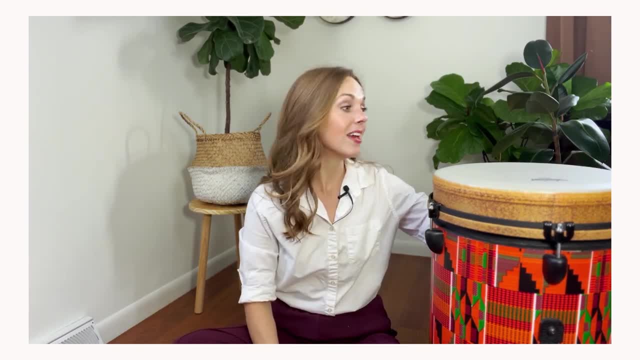 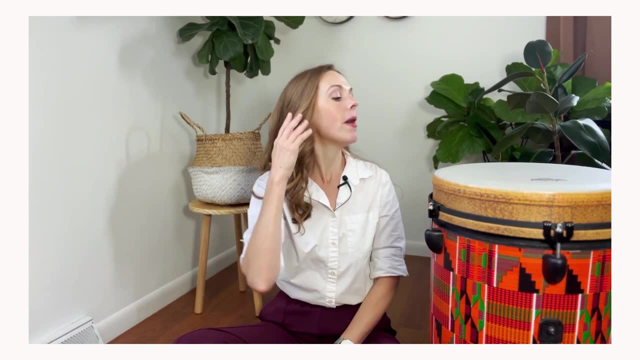 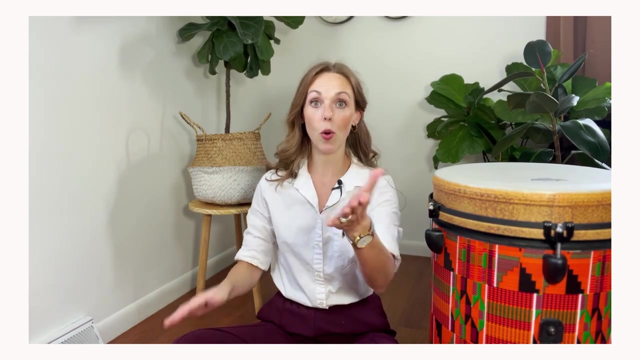 And next to Xander might be Rachel. My name is Rachel, Your name is Rachel. So I'm going to guide the class through who is speaking and who is responding, by gesturing to them and kind of speaking everyone's for them. Let's try it. My name is Miss Victoria, Your My name is Jacqueline. 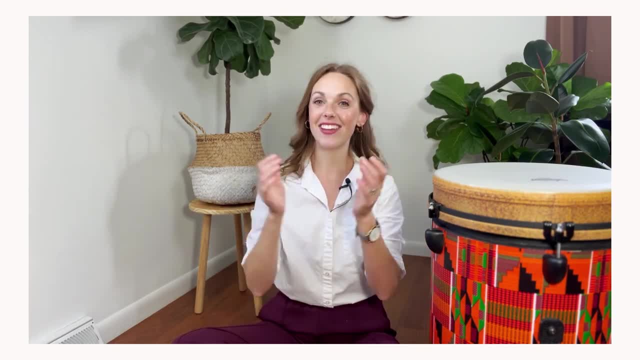 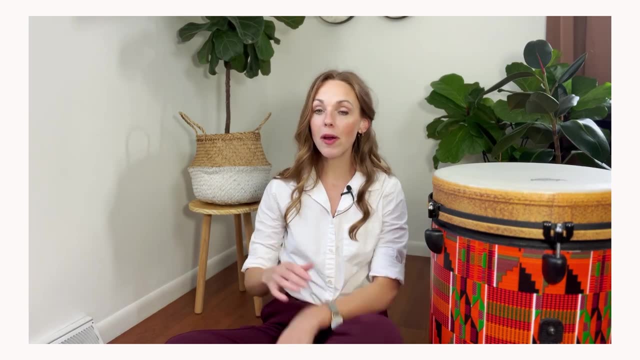 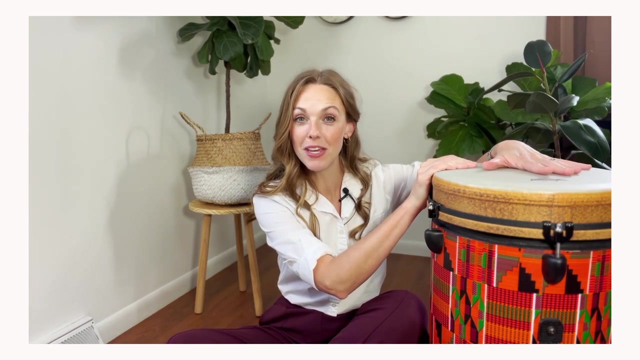 Your. My name is Xander, Your. My name is Rachel, Your. So we're going to go around the circle with people sharing their names, four people at a time. We are playing a drum or some sort of beat keeping device. Everyone else in the circle seated with their 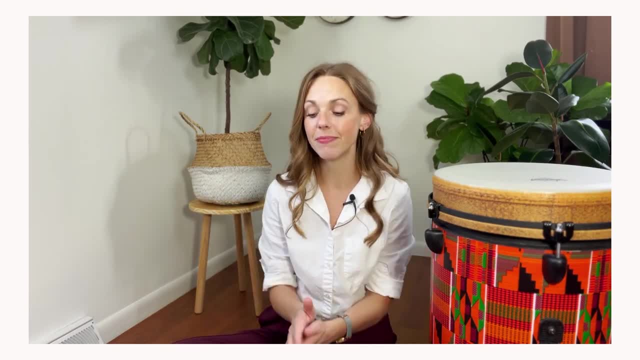 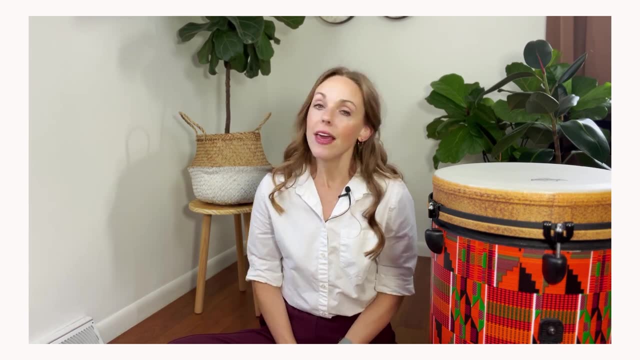 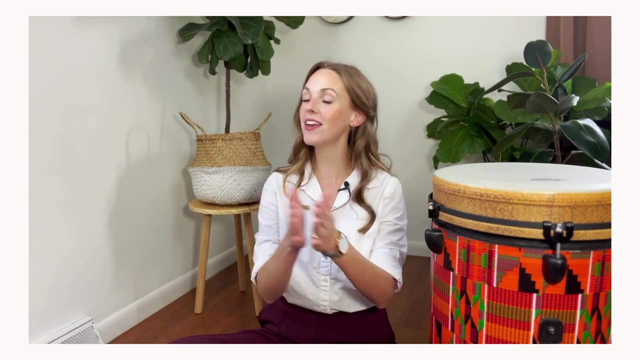 partner. they are doing whatever body percussion motion that they did Now, whatever body percussion pattern that they created with their partner, you know, five minutes ago or so. If you sense that the body percussion thing is not working, then it just turns into this: Everybody does this pattern. 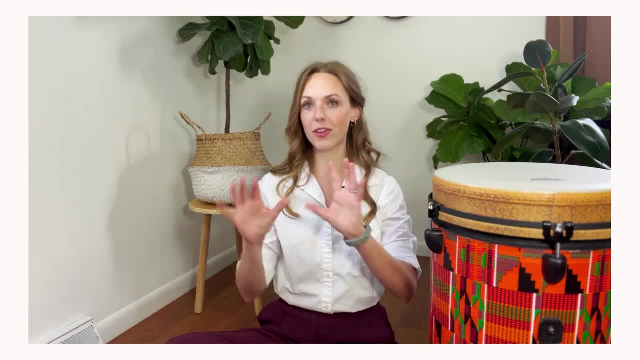 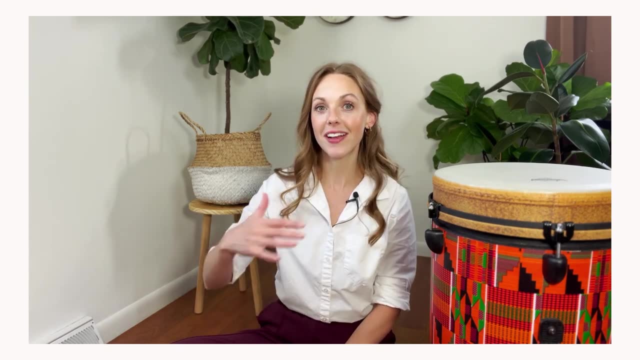 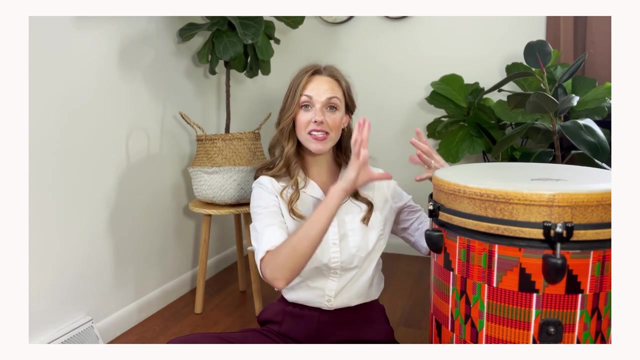 So they still create the pattern with their partner, but then we will transition to everyone just doing the same exact thing, Right? So definitely um several different layers of complexity that we can add to this, just depending on what students need at the time. The idea, though, is that they've had some sort of 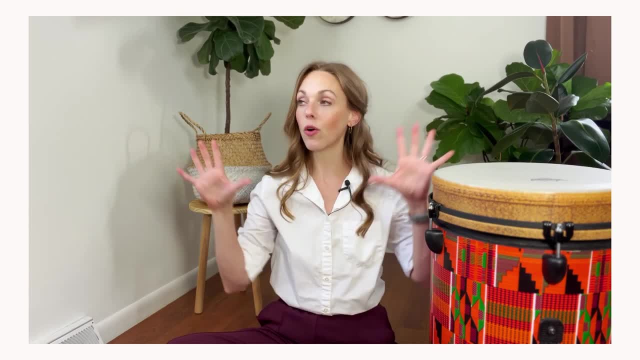 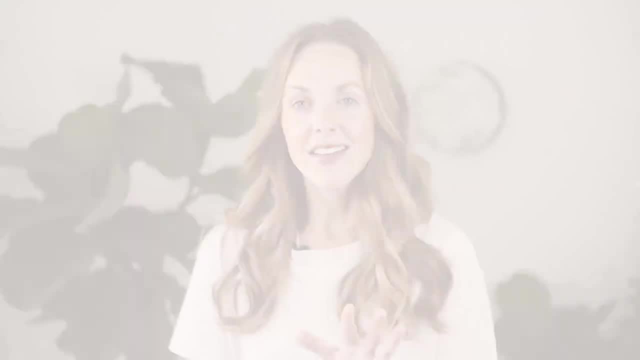 creative body percussion invitation that they've done with their partner. We're all seated in a circle. We speak up the ladder, down the ladder, students go around four at a time and share their names. Let's talk about this idea of open space. Open space is a really important concept because 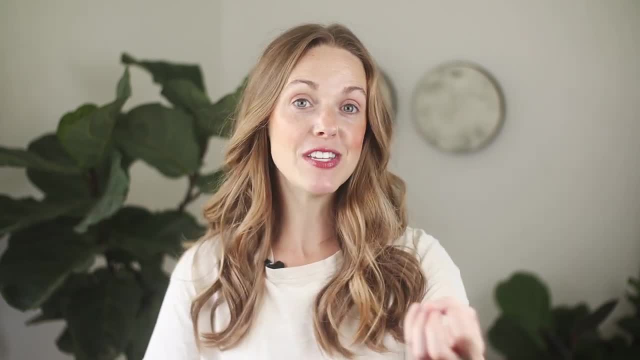 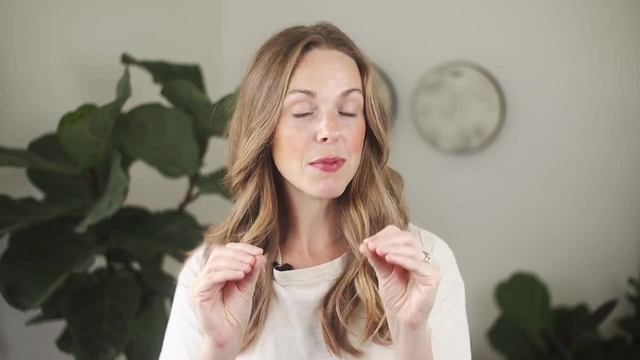 it's how we keep each other safe As we move throughout the physical space of the music room. So we've talked about lower, we've talked about upper. Now let's zoom to middle elementary in the planning binder. This activity is for second and third grade. 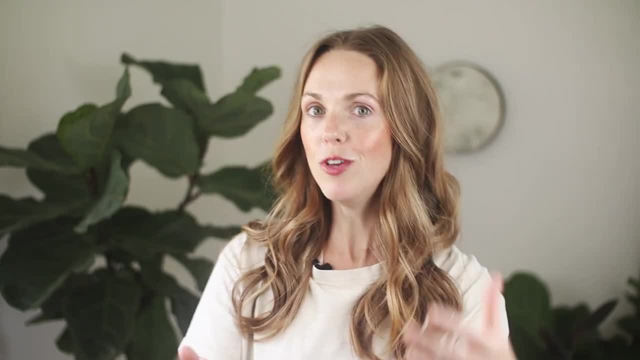 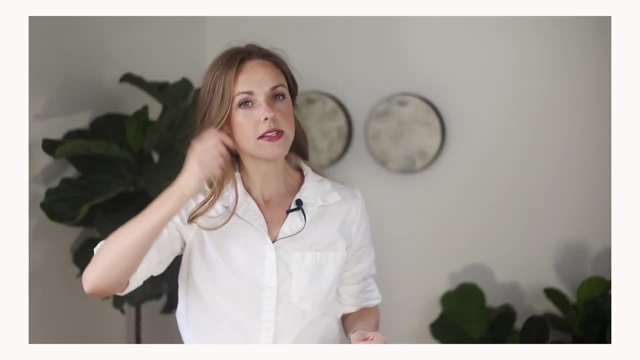 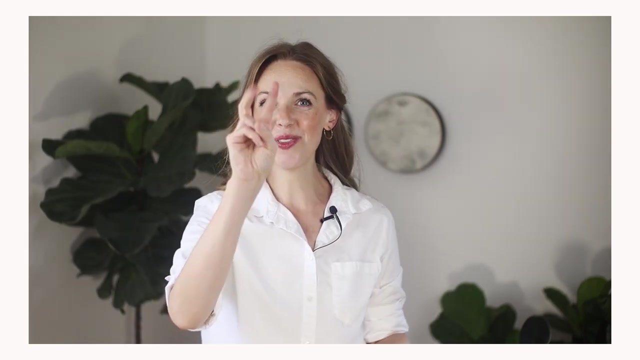 So let's talk about, uh, introducing or reviewing this idea of how we use our physical bodies in the learning environment. Will you copy my motions? Your voice is off, Your ears are on, your bodies are copying me like frozen, like a statue. 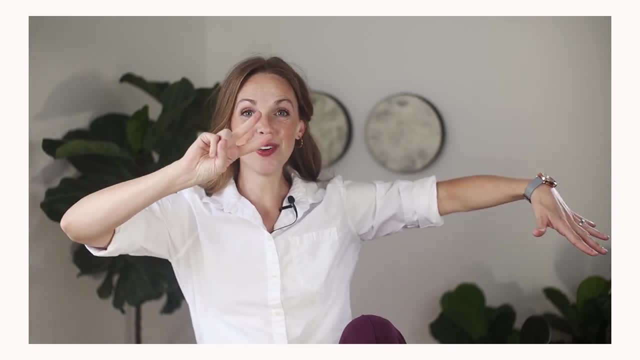 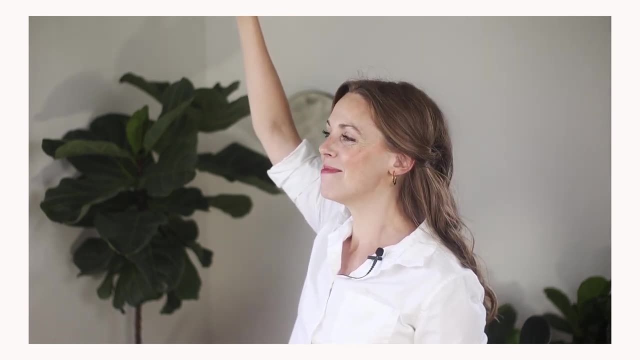 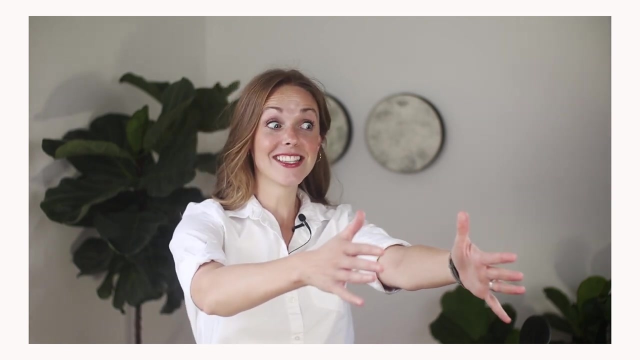 All of the start to absolutely my fear or no thought in a 3. All of the start to the theme like fear. All of the start to the theme my fear, oh, no to like. oh see, Great. So we can go through several rounds of that. What are you doing? 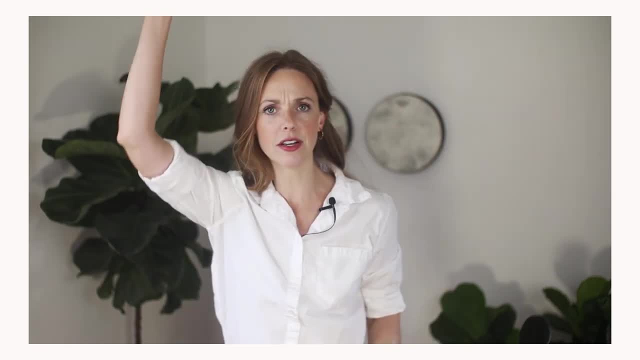 Great, So we can go through several rounds of that. What are you doing? Great. What are you doing? you notice about our song and answers are going to be divergent. we're going to use whatever classroom signal we have for students to wait for their turn to talk, for all of us probably is going. 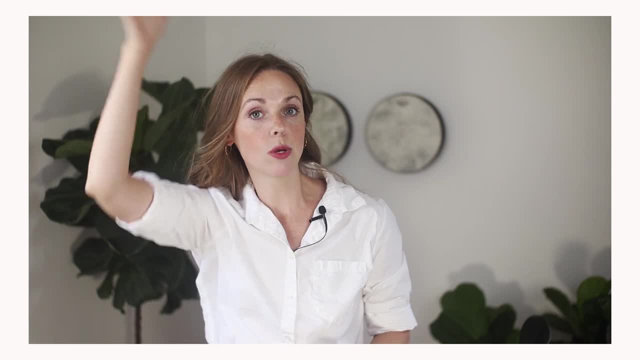 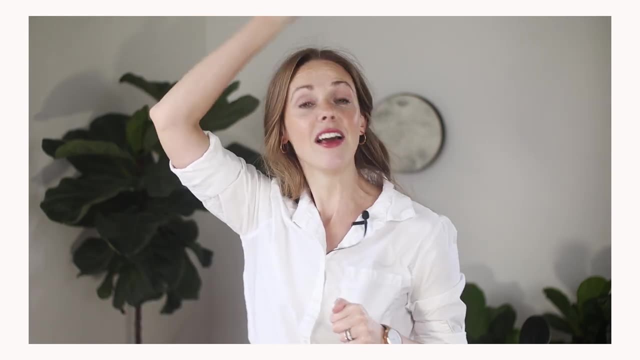 to be your hand in the air, and that needs to be a silent hand. so if your hand is in the air and you're talking to your neighbor, that's not a silent hand, which means i cannot call on you, right? so show me your silent hand that you have something to share, that's something that you 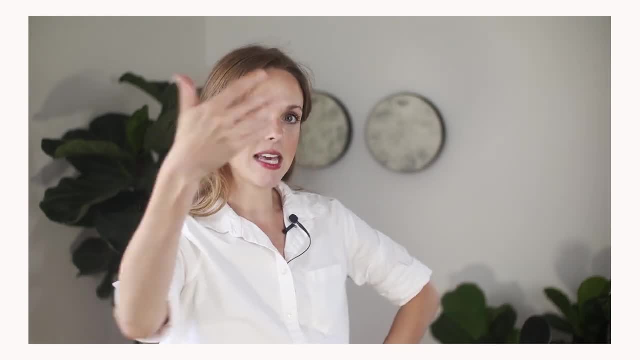 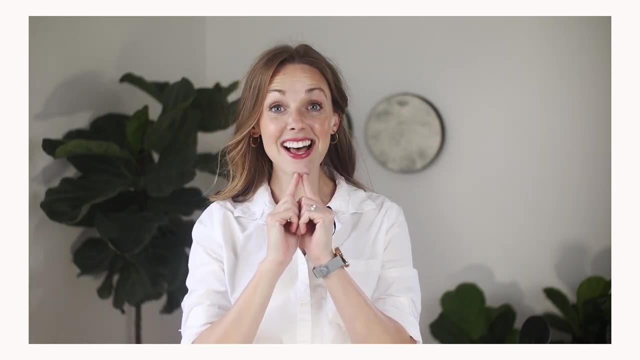 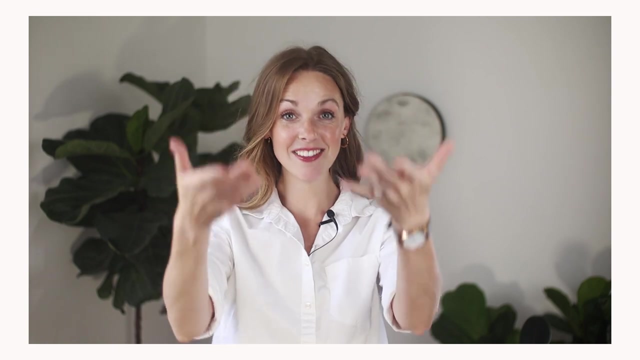 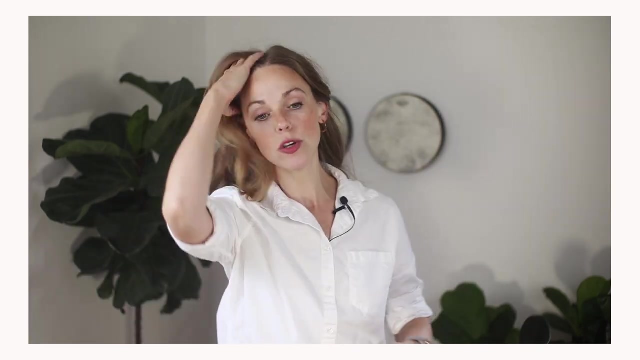 notice. this time i'm going to ask students to sing the second half of the song. they've heard it several, several, several different times: one and two and three. like this. this time, could you do your own statue pose? you may do anything that is safe and musical and school appropriate. now here's. 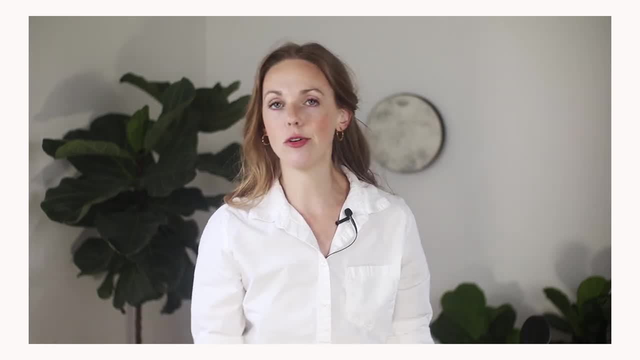 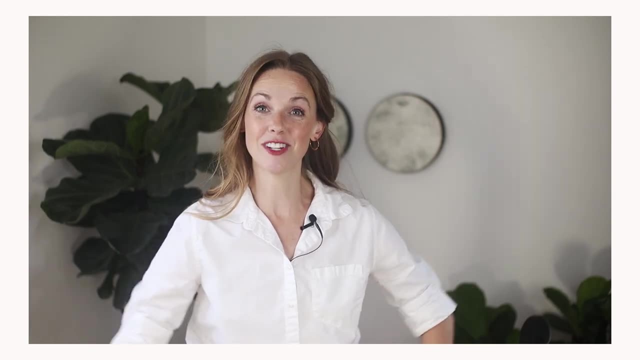 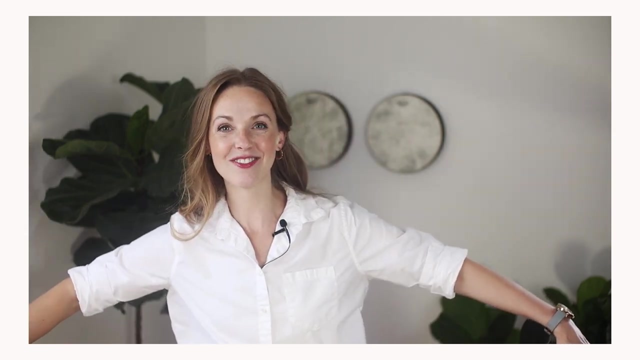 the key. if you follow down, oh then you cannot be a statue, you in our statue garden, so make sure it's a pose that you can balance if you choose to use it with one foot frozen. students are singing the second half. i'm not going to sing with them. 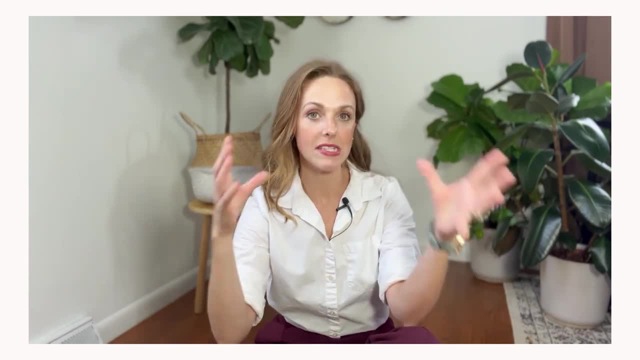 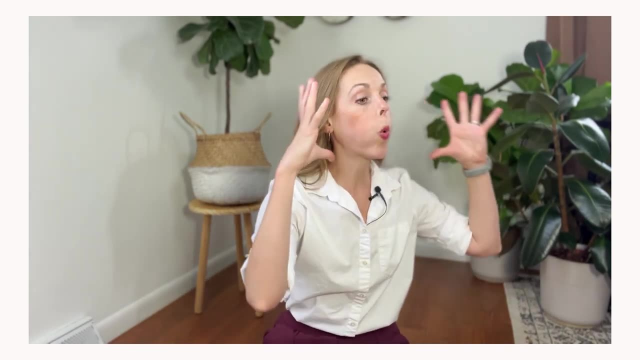 excellent. this is our time to have our open space discussion, so we're going to look around the room for areas that have open spaces space. i'm going to ask a few students at a time to blow a bubble around their bodies and move around the room while we sing. 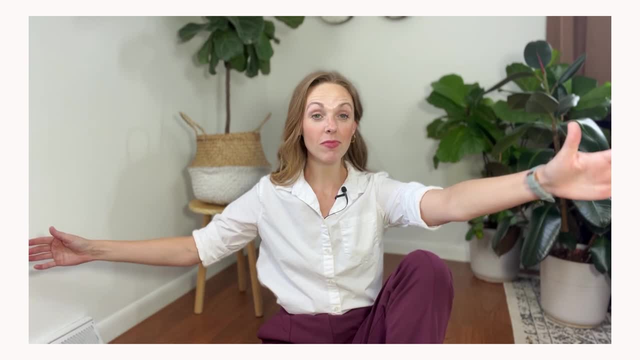 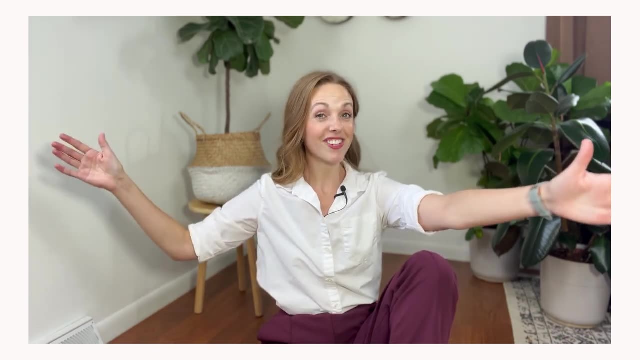 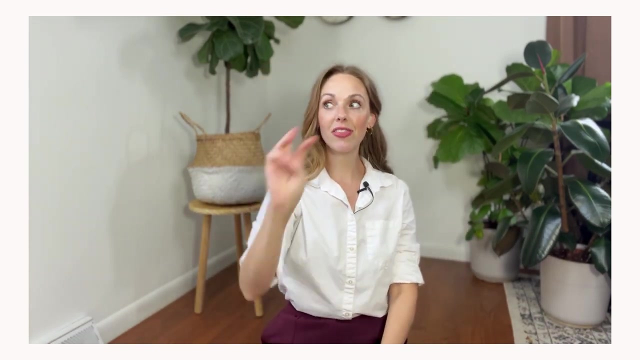 and they're frozen in open space. and then, as a class, we can decide: yes, they are in open space. i'm not sure if they are or no. they are not in open space. we'll give them another shot here. they go moving around, what's that? three, three, and they're frozen in open space. same thing: yes, they're in open space and we're. 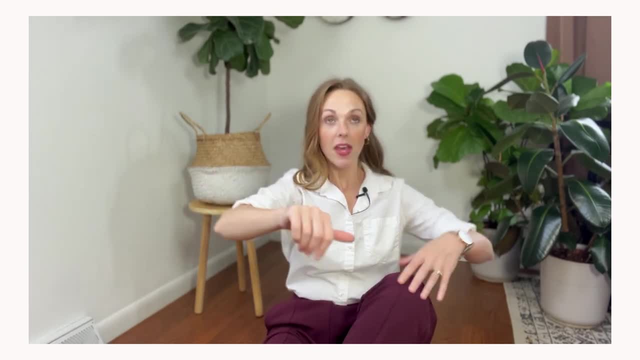 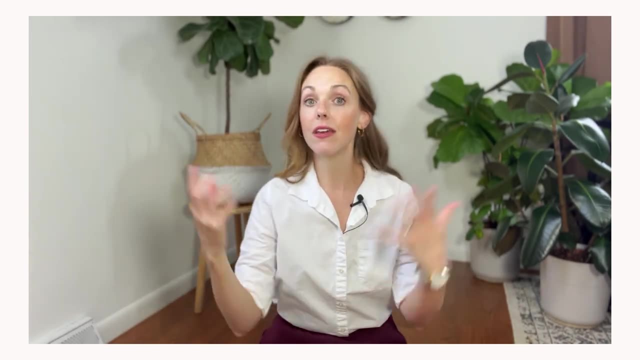 not really sure if that counts as open space or no. they're not in open space. they come back. i'm going to choose another group of students to blow a bubble around their bodies. they go around and do the activity eventually, either in this class, if these are students who already know all about. 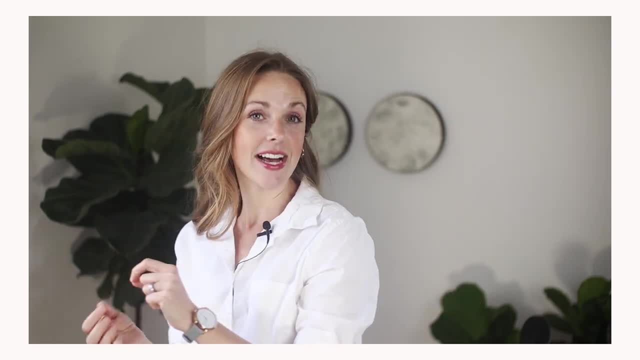 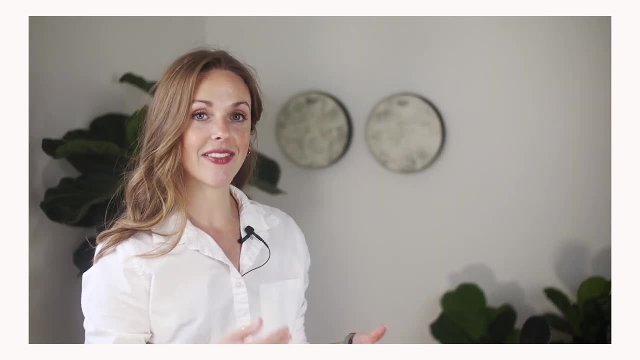 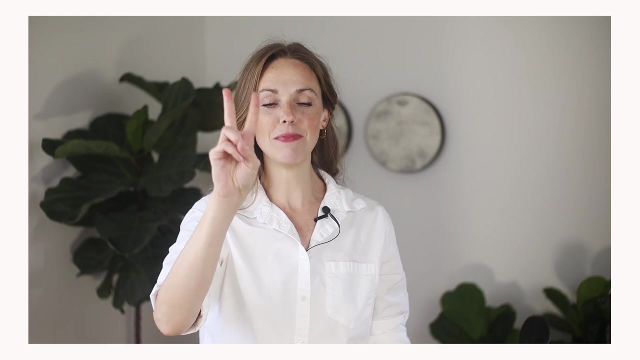 open space- and this is just review- or in the next class. however, you know the the time works out. in the next class, everyone is walking around the room in open space and at the end, your statue needs to be frozen and you need to be in open space. if you are not frozen and if